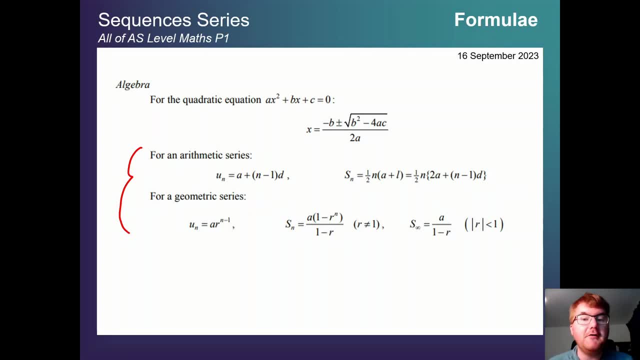 get certain formulae and for this video in particular it's very important to know these particular formulae. Just one point to make here. I also use the other version here. so SN equals A brackets R to the power of N minus 1 over R minus 1.. You may have been taught that. 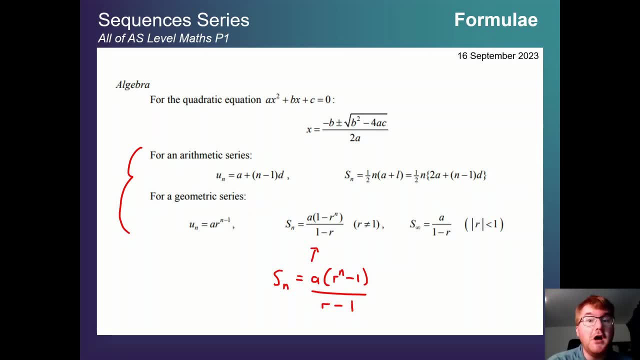 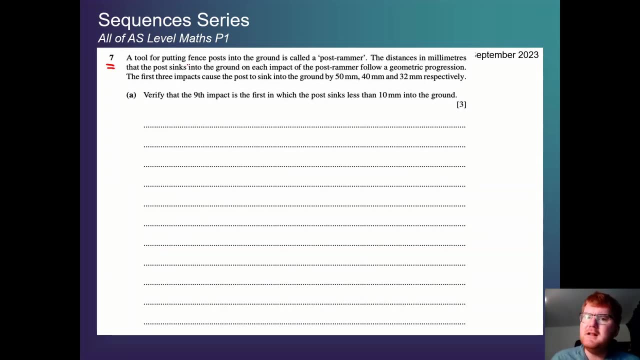 in class as well. so it's important to realise you have that alternative. All right, let's get started. So we have question 7 here, so slightly more on the difficult side, and we've got a little bit of word worded question here. So when we have this again, just take your time, look through the 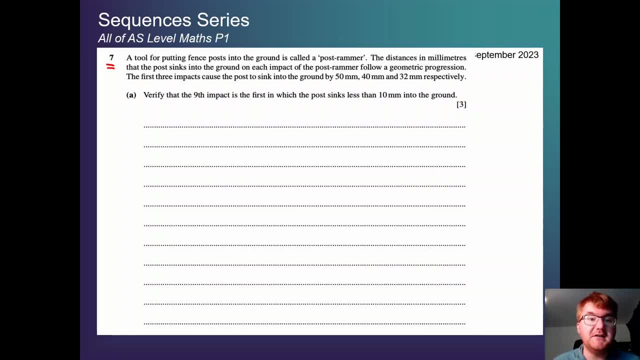 question and then make sure we are answering everything for the three marks. So a tool for putting fence posts into the ground. it's called a post rounder, Not particularly important, but again, give us some context, The distances in millimetres. that's important that the post sinks into the ground on each impact of the post. rammer follows a geometric 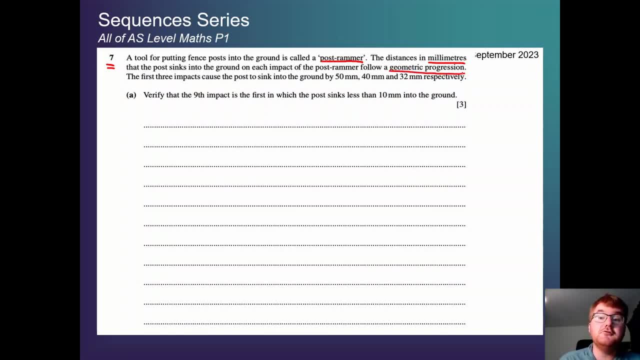 progression. So whenever I'm doing a sequence and series or progression question, I want to identify: is it geometric, so multiplying each time, or arithmetic, which is then adding or subtracting? So this is going to be multiplying. so keep that in mind and the first three impacts cause the post. 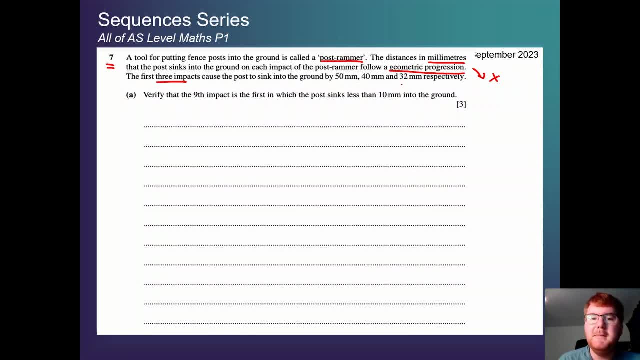 to sink into the ground. So this is going to be multiplying, so keep that in mind. and the first three impacts cause the post to sink into the ground by 50, 40 and 32 milimetres. So essentially we have a sequence here that goes 50, 40 and 32.. 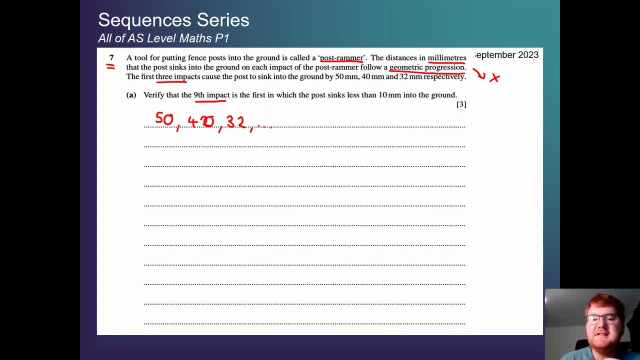 And we need to verify that the ninth impact is the first in which the post sinks less than 10 milimetres into the ground. So soon as I see a sequence and I see geometric, I need to be thinking right. what do I need to work out? to work out the nth term, And in this case we need the first term. 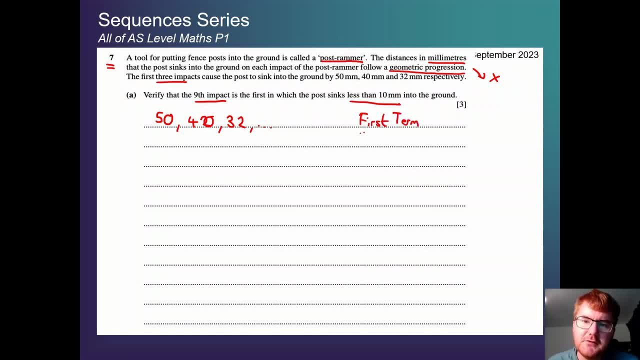 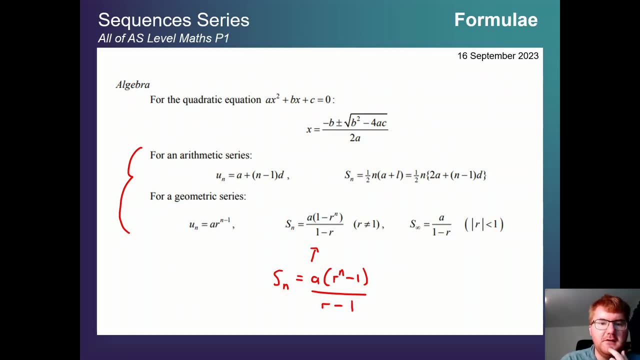 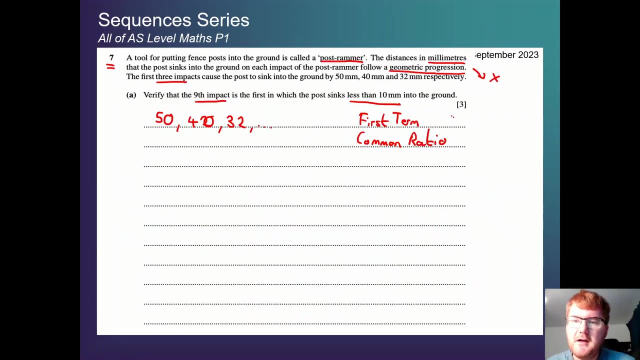 for a geometric progression and what's called the common ratio. then we can apply our nth term formula to that. so notice here, we actually have this formula on the formula sheet, so we're going to come back to that in a moment, but we need to find this first term a and common ratio r. now the 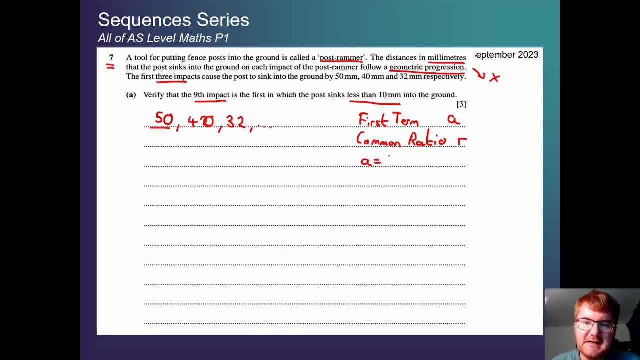 first term is really straightforward. we're already told this. so a is equal to 50. to work out the common ratio, all we need to do here is take, for example, the second term, so 40 divided by the first term. or we could take the third term and divide that by the second term, so it's the term afterwards. 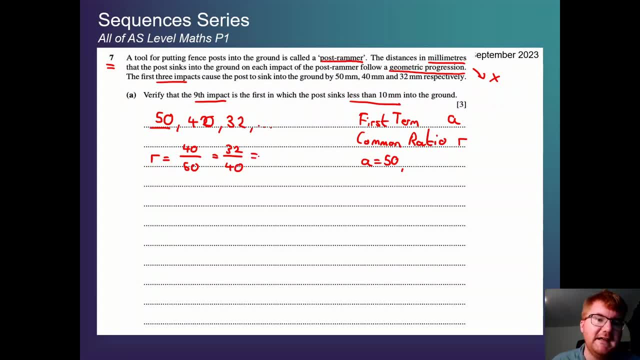 divided by the term four. if we pop that into our calculator or simplify the fraction, we will then get 0.8.. So now we now know what a is the first term and the common ratio, so what we're multiplying, we get 0.8.. Now we know the common ratio, so what? siis? this is a tall order equation. 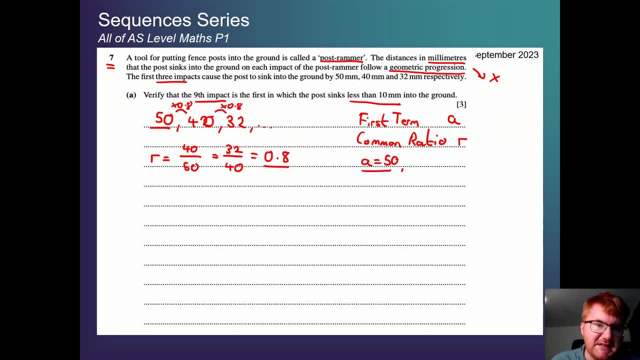 by each time, in this case, times 0.8. we can then write down the nth term. Now, all I'm going to do is I'm going to copy down this formula. so ar to the power of m minus 1. wherever I see an, a, I'm. 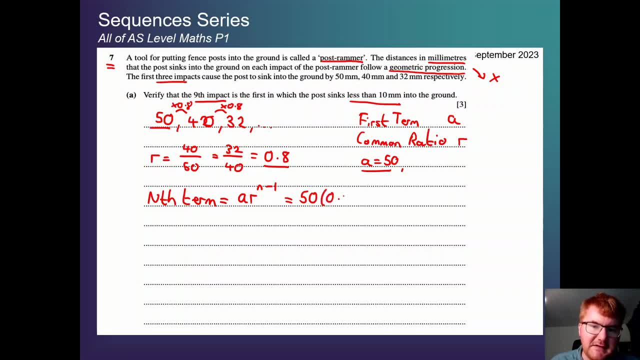 going to put a 50. wherever I see an r, I'm going to put a 0.8.. So this is the formula that represents to work out anything in the particular sequence. Now it wants us to think about the ninth impact. so I want to work out this nth term when n is equal to 9.. So when n is equal to 9, we pop this. 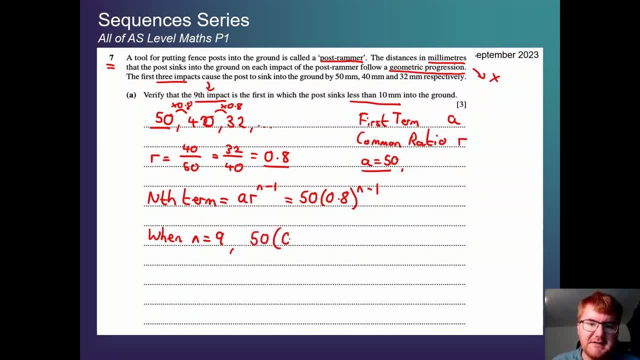 into the formula. so we have 50 open bracket, 0.8 to the power of 9 minus 1, and I'll just pop that into my calculator. so make sure you've got your calculator handy here- and we should get 8.38 dot, dot, dot. and this is in millimeters and certainly this is less than 10. 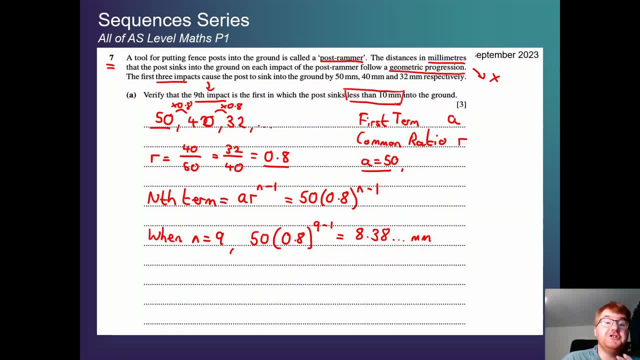 millimeters. so we're going to have to work out the nth term when n is equal to 9.. So when n is equal to 9, that's going to be less than 10 millimeters into the ground. However, we're not finished here, because we need to check when n is equal to 8, so the term before, and just ensure. 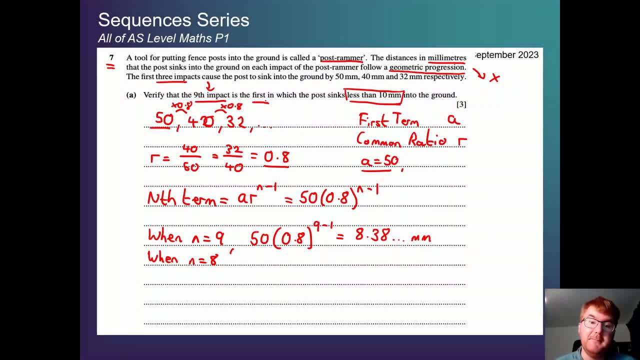 that that is above 10. so therefore it is the first in which it goes less than 10 millimeters. So to get the full marks on this question is a little bit sneaky. we also need to check when n is 8. so very similar calculation, just 8 rather than 9.. If I pop that into my calculator, I then get: 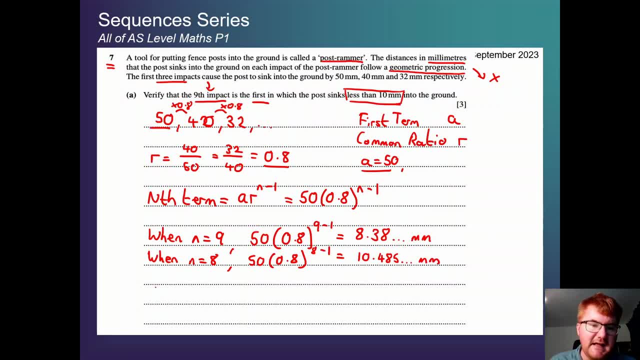 four, eight, five, dot, dot, dot millimetres and therefore ninth impact- I'm just going to write this as a sentence- is the first below 10 millimetres. So notice, here again, I'm taking this question very seriously and making sure I'm getting all the marks by checking. 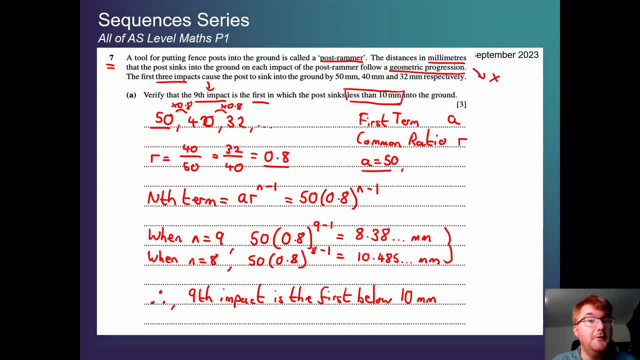 the n is eight and making sure that that is not below the 10 millimetres. If it was, for whatever reason, I would then check my working and make sure do I have the correct first term? Do I have the correct ratio as well? Now on to the next two parts of the question. 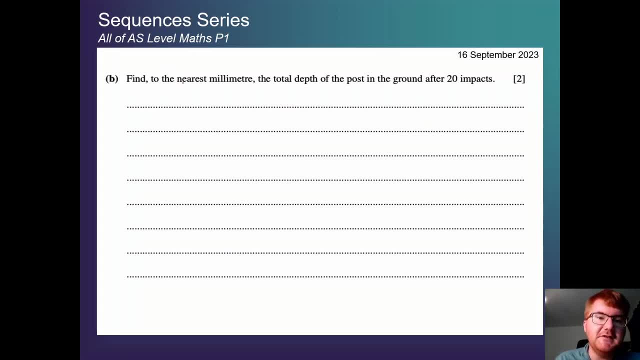 which are much more standard, And the first thing find to the nearest millimetre. So notice the rounding that we have to do here. The total depth of the post after 20 impacts. As soon as I see total in any question, I am thinking the sum formula. Now remember. 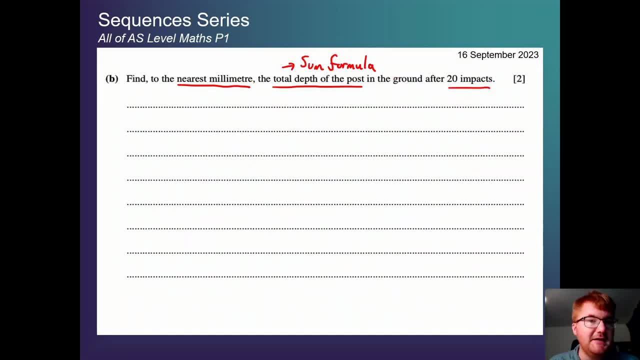 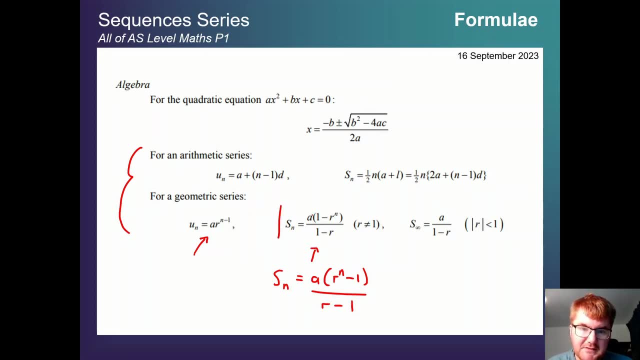 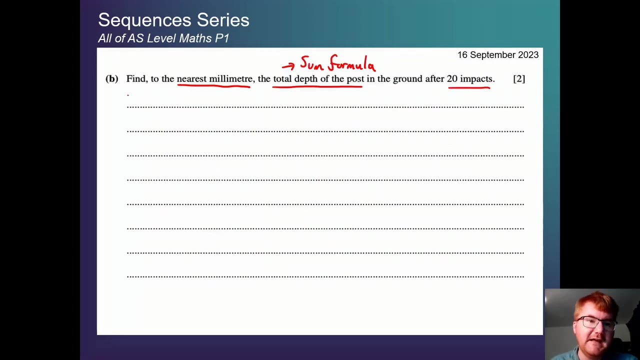 from before. We're looking at geometric here, not arithmetic. So I go back to my formula and go: okay, I want to use the geometric series formula, So I'm going to be using this one- Notice how I've broken that down to find the correct formula. So if I write this formula down, 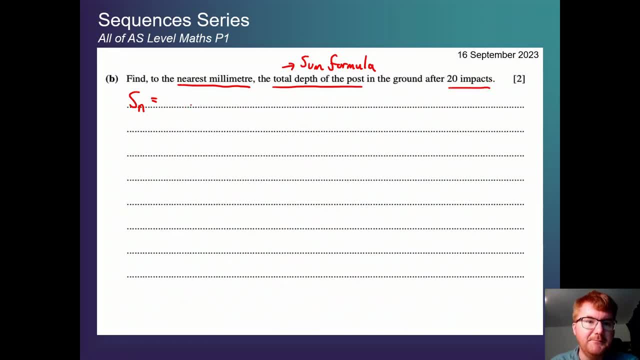 just don't have to do this in the exam, but just so I've got it here. then we can use either formula: Absolutely fine. So a brackets one minus r to the power of n over one minus r. We're just substituting our values, So a, the first term was equal to 50 here The common. 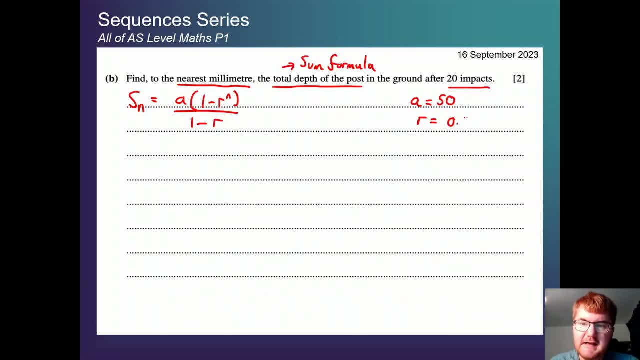 ratio was equal to 0.8.. And then we just pop this in, So we're looking for s20.. So notice: n here is equal to 20, because we have 20 impacts. So then we pop in 50, open brackets. 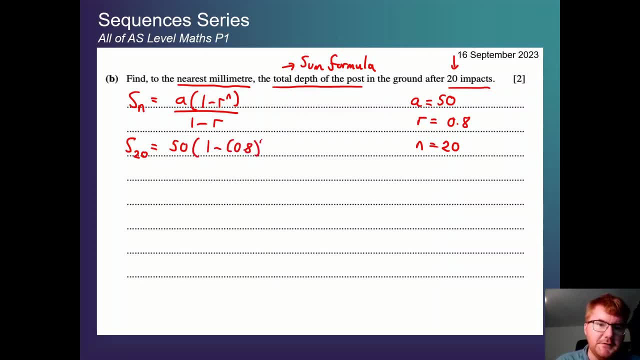 one minus 0.8 to the power of n. However, we now know n, So we pop in 20.. There we are, And then we have over one minus 0.8.. And this is now just a calculator exercise. Make sure, when you're typing this in, you're very, very careful. 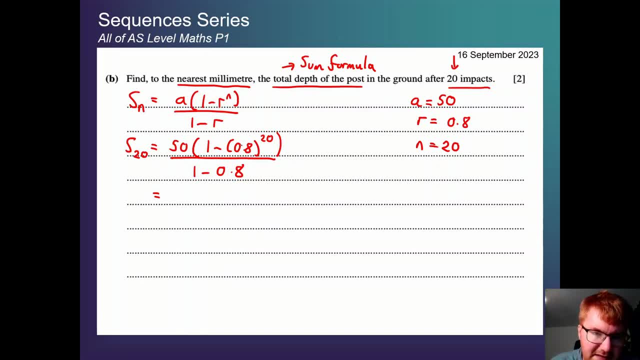 making sure you put the brackets in the right place. Notice, there is a decimal point here, And if you put this in correctly, you'll then get the answer of 247.117 dot dot dot. However, this is where we want to pick up that second. 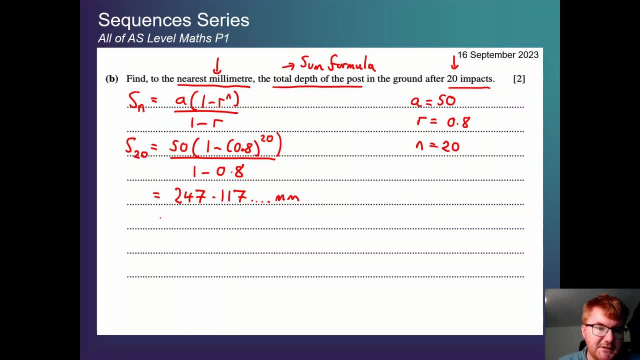 Mark to the nearest millimeter. Read that question. So we just want to round this then to 247 millimeters to nearest millimeter. So very important. Read the question. This will change sometimes, So you do need to make sure you're putting down the precise answer. 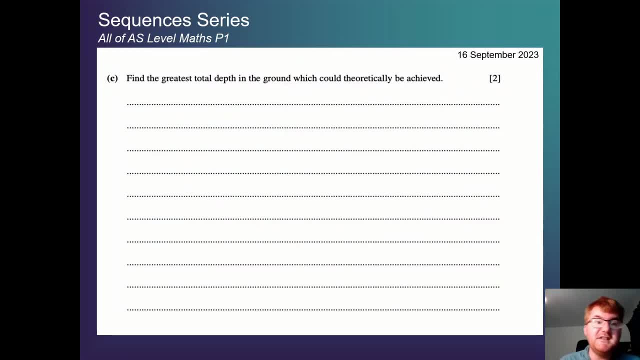 for those two marks. Now question C again is also a classic. I see a particular word or phrase and it triggers something in my mind here. So here we have: Find the greatest, That's important, Total depth in the ground which could theoretically 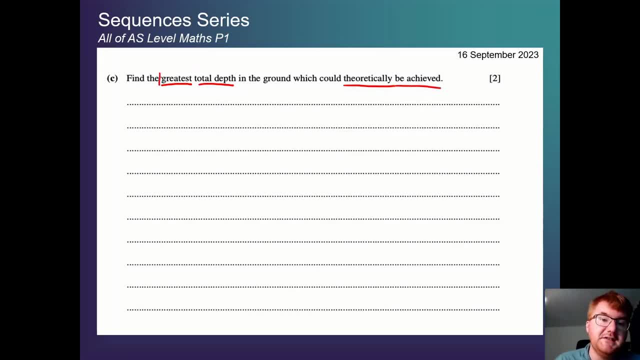 be achieved. So as soon as I see a phrase like greatest or I see a phrase like theoretically could be achieved, I'm already thinking to myself: the sum to infinity formula, That's the first thing that goes into my head here. If I go back, we have the sum to infinity. 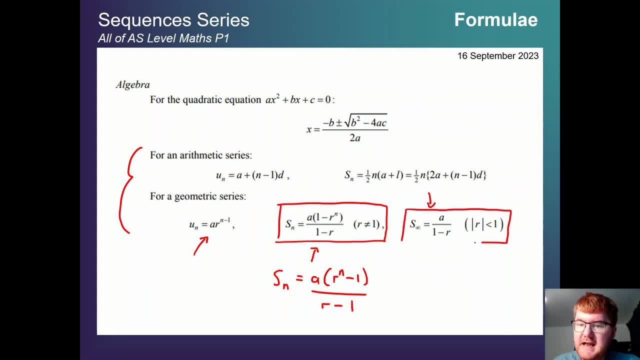 formula here, just right over here, which is equal to a over one minus R. And notice: the magnitude or the Modulus of R needs to be less than one. Notice: in this question we have R is zero point eight. So that does fit the condition. Therefore we are allowed to use that formula. So I'm. 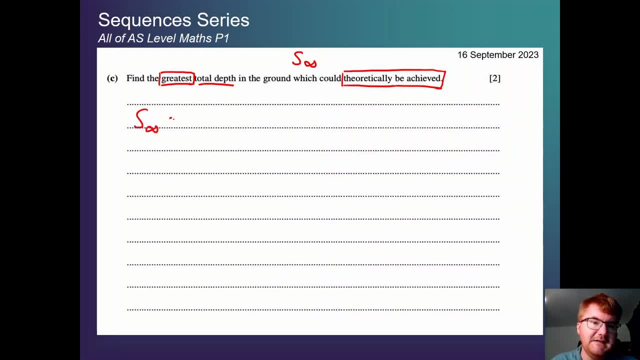 going to copy it across. So S infinity Is equal to a over one minus R. And notice again, we've got a is equal to 50, and double check these things in the exam. R is equal to zero point eight. So we pop it into our 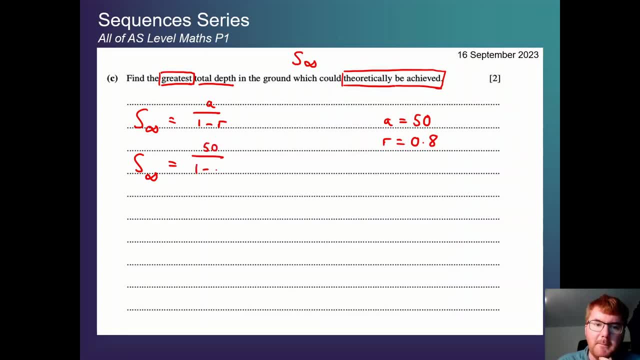 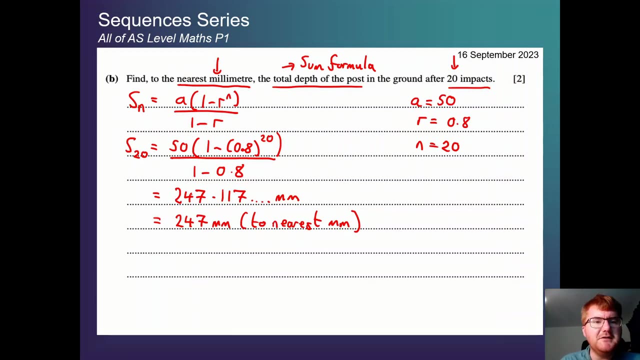 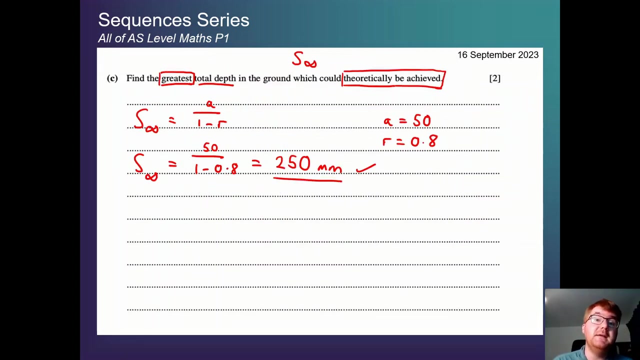 formula. So we have 50 over one minus zero point eight, And then that's equal to 250 millimetres, which is our correct answer- Notice in the context of the question. So we go back to what we worked out. after 20 impacts We had 247 millimetres. So the answer of 250 millimetres. 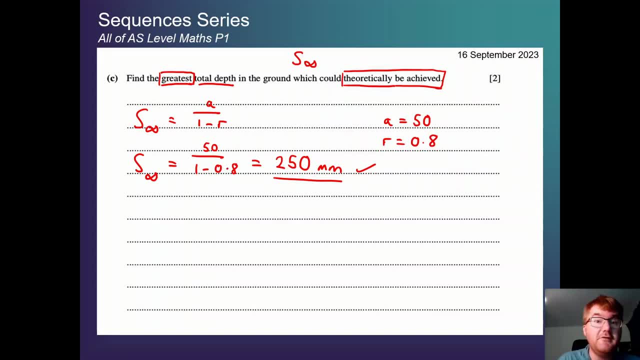 makes a lot of conceptual sense. It should be a little bit more than 247, but not that much more. So with that we now have to look further in and find our answer. Alright, so who has got a higher score to work with? 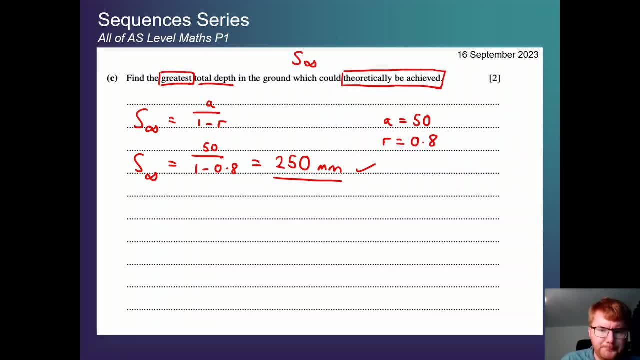 In case we could even pick one method. Yeah, maybe you could ask the question. So the answer is yes, but if R is zero, then you're using the wrong method. So then you could have one method and you'd be converging quite quickly to the theoretical. 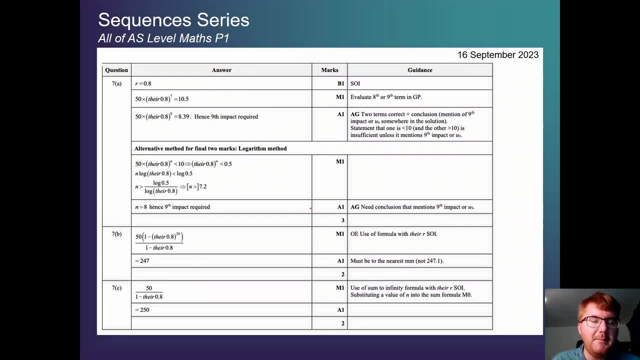 greatest total depth. Again, you can have a look through the answers here and you can see where we picked up the method mark. I've taken this approach of part a. again, you could use logarithms. That is absolutely fine as well. 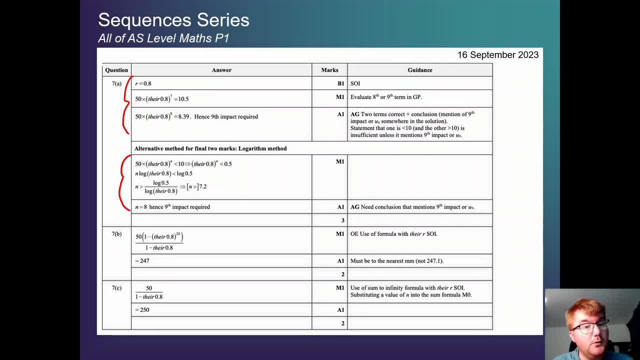 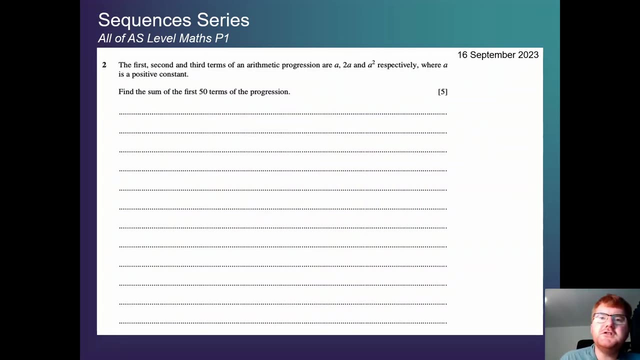 And then kind of solve the equation at this point and then look at an inequality. that is absolutely fine as well. But just be aware that this approach here that I took, which I think is a bit more common sense approach, also perfectly fine as well. okay, on to a very different style of question. it is earlier in the 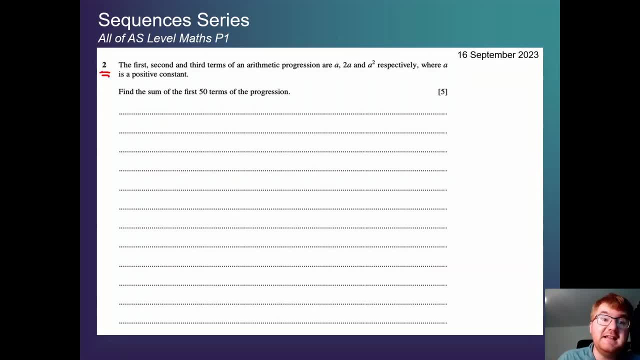 paper. so on the surface it should be more easy to do, but it's less structure in this kind of question and this can come up and i'm going to show you how i think about this question. so we have the first, second and third terms of an arithmetic progression. i see that key phrase. 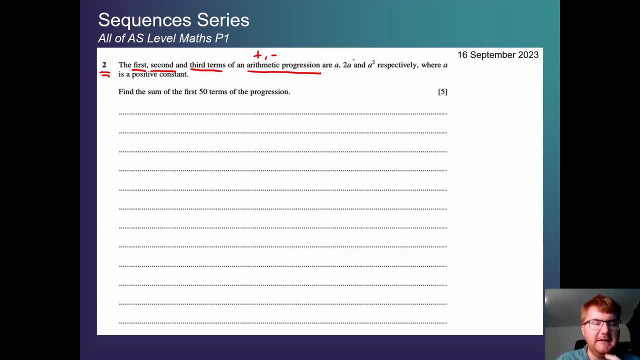 so we're going to be adding or minusing in our particular progression that we've got here and we have a to a and a squared where a is a positive constant. that's more important than we think as we go through the question and we want to find the sum of the first 50 terms of the progression. 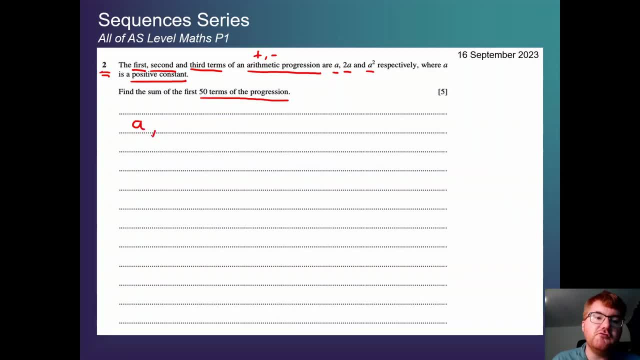 okay, so the first thing i'm going to do is just write down the progression a to a and a squared. now notice: this is arithmetic, which means we're either adding or subtracting, and whenever we're talking about arithmetic progressions, when you talk about the first term, well, that's just equal to a. anyway, that's kind. 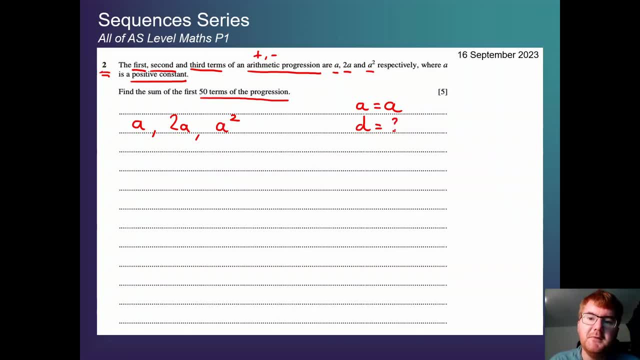 of convenient, but we do need to work out this common difference here. now. some students. they see a question like this and they think there are no numbers. there's no numbers. how could i even work something out without any numbers? however, let's just follow the idea for a common difference. 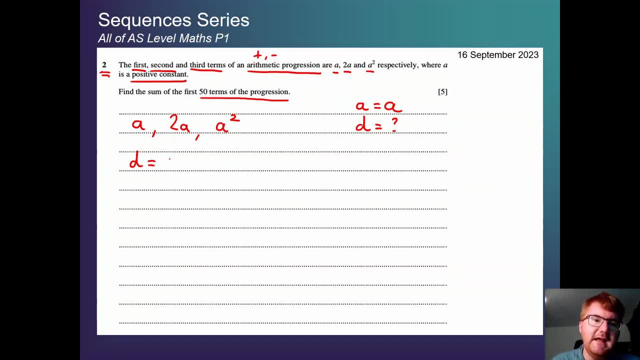 to work out the common difference. all you need to do here is to work out the common difference and then you can work out the common difference. if you just look at the tells us the common difference between a squared and a squared, so that we got a squared as the common denominator. we'll take c, squaredhcdbdhcd, and provided: 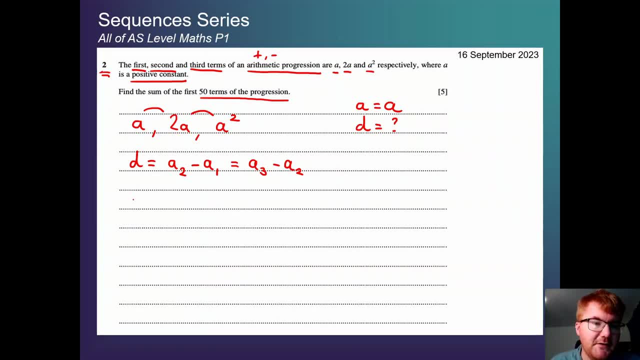 that what we've done by doing this. so the first term is a squaredhcdbdhcdbd and Decimätron, even though we didn't write each first term, so this will do so. it's going to listen to the second term minus 2a and because both of these things are equal to the common difference, these two things- 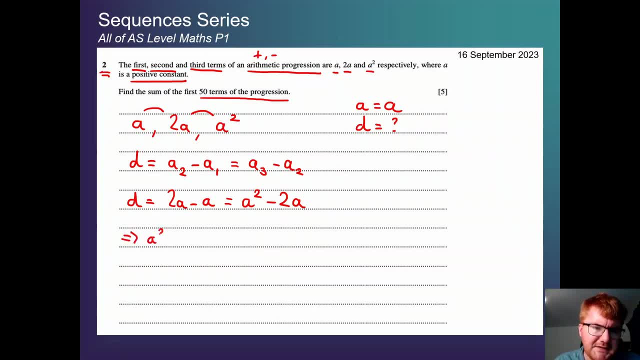 must be equal to each other. therefore, a squared minus 2a is equal to 2a minus a. still feels like at this point we're not going to get a number out of this, but keep the faith, we're going to go through this now. so, first of all, we can just simplify the right hand side: 2a minus a is just. 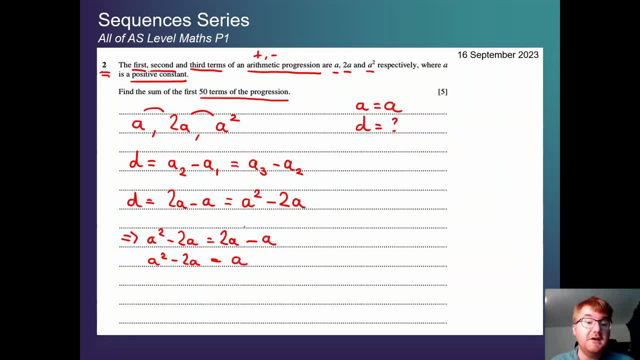 a, then we're going to bring everything to the left hand side because- notice, here, let's do this in a different color- we have a quadratic, yeah, so, even though this is not a quadratics video, if you want to check out my quadratics video, of course, you can always go to the playlist. 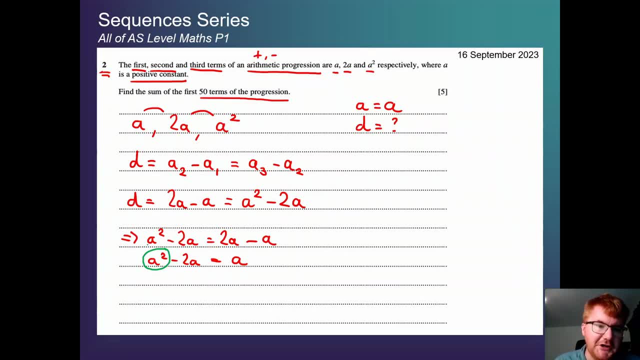 and find quadratics there. but notice we're using other knowledge from the course, so we are using quadratics here and that knowledge as well. so what we need to do then is go minus a from both sides. that can gives us a squared. squared minus 3a is equal to 0. And this is actually a very straightforward quadratic here. 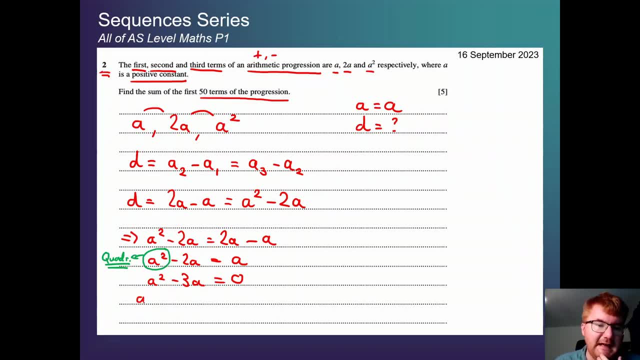 to solve. We have a common factor of a, So we take a out, Then we work backwards. So what do we multiply a by to get a squared a? What do we multiply a by to get minus 3a, Minus 3.. And if two? 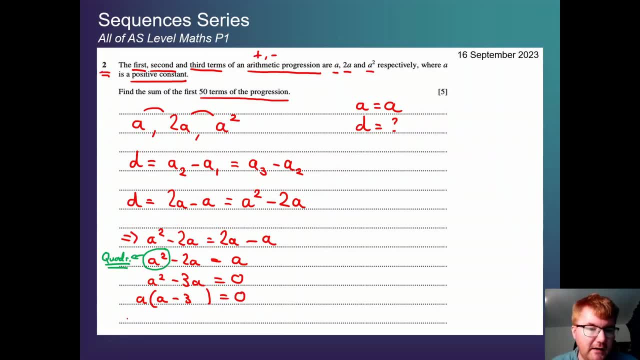 things. multiply to give you 0,. I'm sure you've heard this a lot. So either a is equal to 0,, so the first part is equal to 0, or the bracket is equal to 0, and therefore a is equal to 3.. 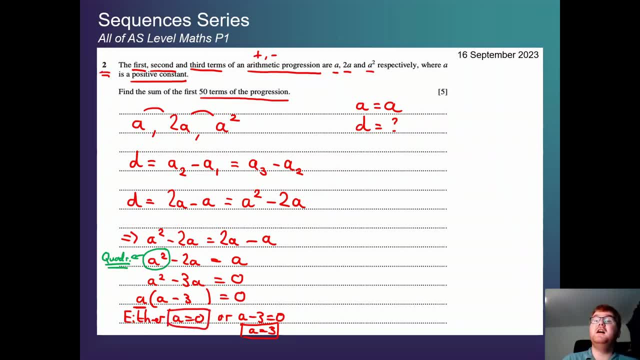 Now notice we have two possible answers. but back to something I underlined already: a is a positive constant. Therefore, 0 is not possible. Therefore a is equal to 3.. Now let's write this question out a little bit differently. Now we know a is equal to 3.. The first term is 3.. The second term 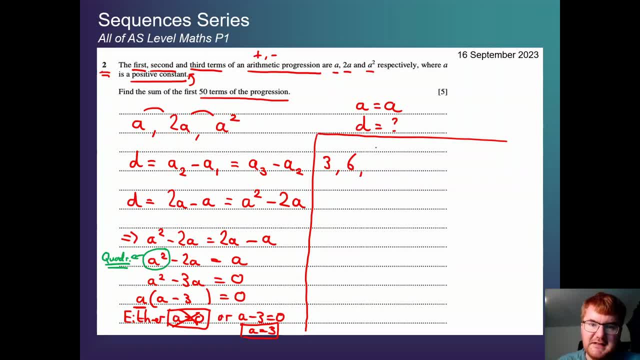 2a times 3 is 6 and 3 squared is equal to 9.. So notice, I'm always double checking as I go through the question here. Do we have an arithmetic progression? Are we adding 3 each time? Yes, we. 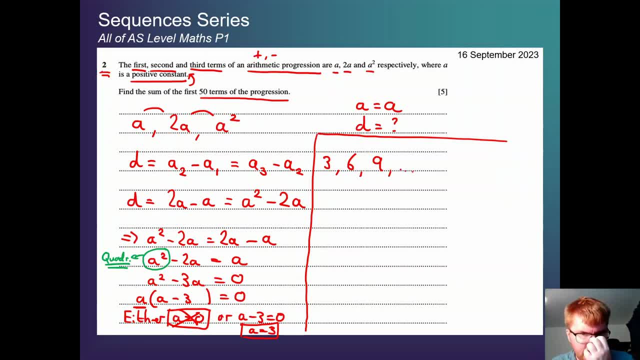 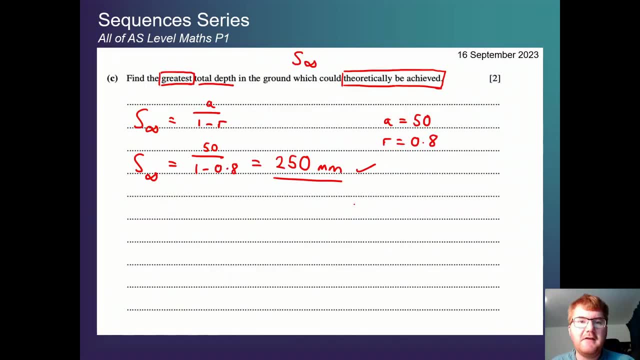 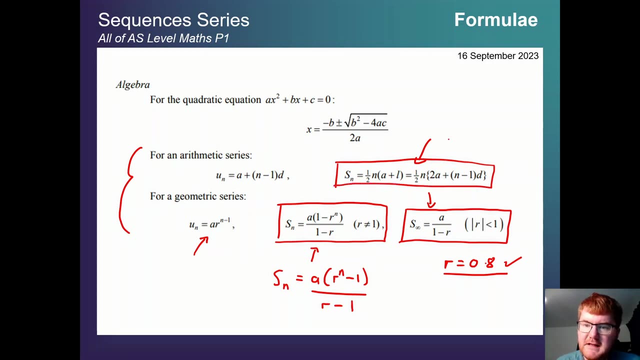 are, So we do have the correct progression. Now we want to find the sum of the first 50 terms, so we're going to use the S50 formula. Notice, this is arithmetic, so we're going to be using this formula over here for an arithmetic series, and specifically this one on the right hand side. 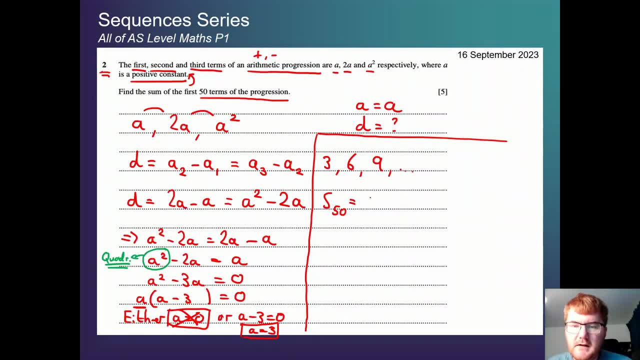 So let's pop this in. So we have n over 2, so n is 50 here, so 50 over 2.. Two lots of the first term, so two lots of 3 plus n minus 1.. Again, n minus 1. 50 minus 1 is 49 times the common difference. 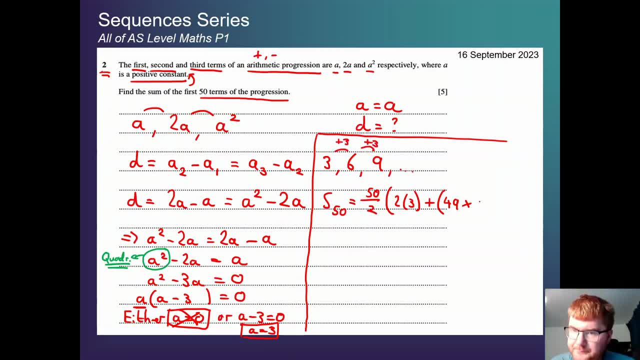 Well, we are adding 3 each time. At this point. you can either do this without a calculator. you can break this down or pop it straight in. I tend to do a mixture of both here. so 50 divided by 2 is 25.. 3 times 2 is 6.. 49 times. 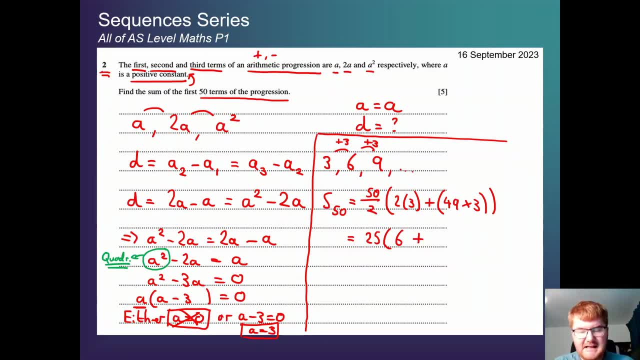 3 again. no need to do this mentally Again in exam pressure. you don't want to be relying on that. and now, if we pop the rest of this into the calculator, we get our final answer of 3,825.. So we've got a total of 3,825.. So we've got a total of 3,825.. So we've got a total of 3,825. 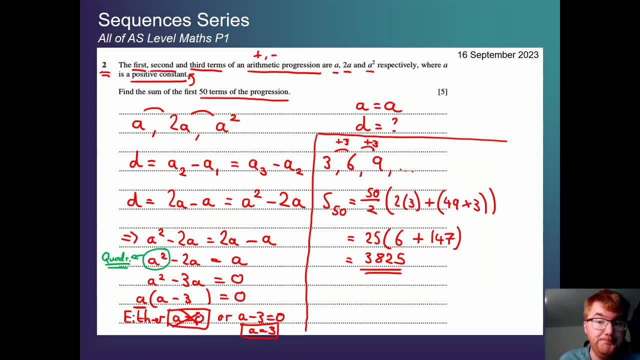 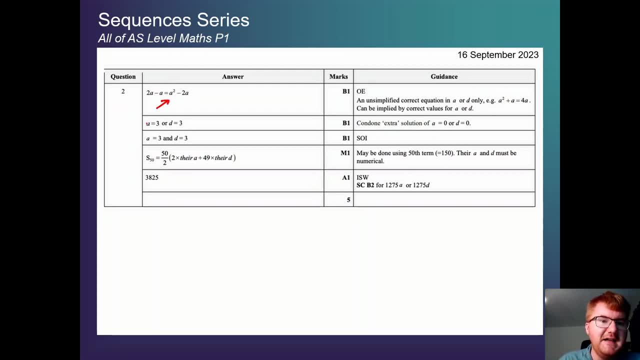 you can add this back in the calculator into our system. Here's the final chunk. so don't forget to keep the three first zeros and pastодen to вотic all five marks. on this particular question, OK, you can have a look through the mark scheme, say where I picked things up. So notice, we've got this. 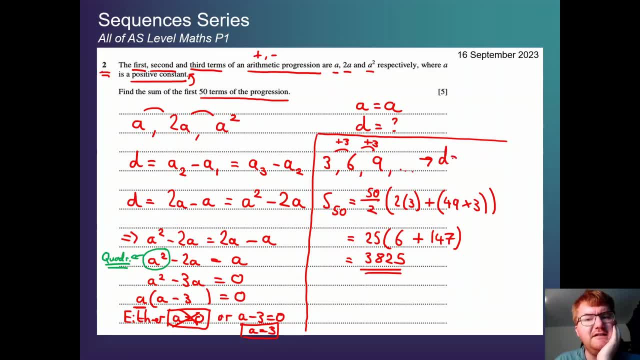 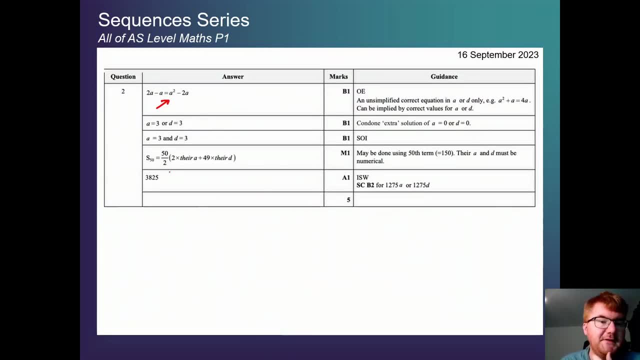 part here I could put a is 3 or d is 3.. So that's interesting, but I didn't explicitly put d is equal to 3.. So possibly at this stage I would write d is equal to 3, just to make sure we're getting that. 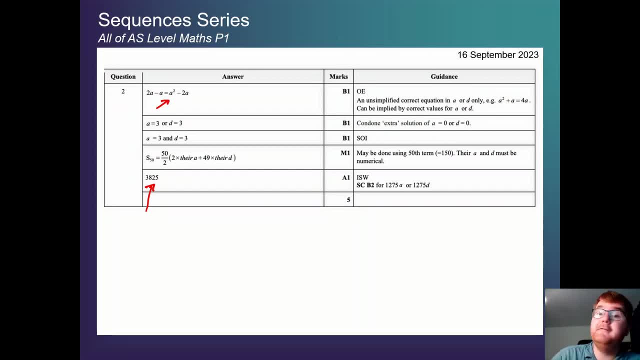 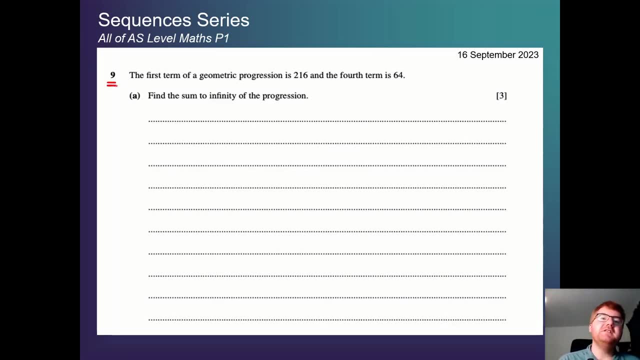 third mark there, So I didn't do this. eight hundred and twenty five, okay, and on to question nine. so a little bit more of a tough question. if you found this so useful to you so far, then please do like and subscribe. that helps the channel go a long way and if you want more of this, a level content, also looking at stats paper. 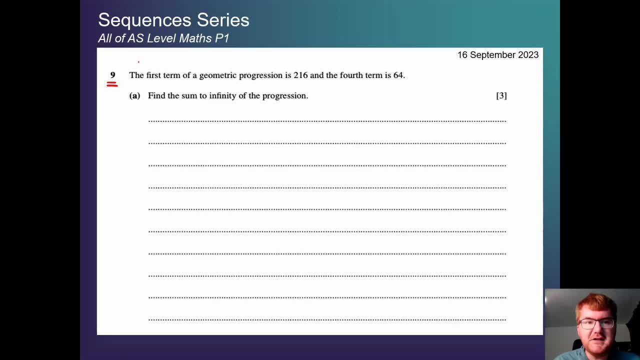 five, then certainly it's something that's in mind. so the first term of a geometric progression- i'm underlying this every single time i see this- is 216, and the fourth term is equal to 64, and from this- we need to find this and we've seen this before in the video- sum to infinity. now let's. 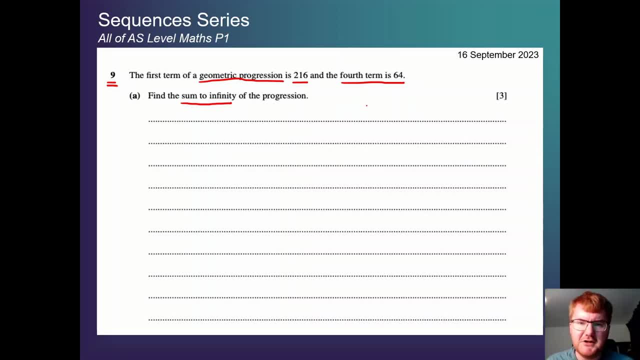 just go through some sort of fundamentals here. if i have a geometric progression, then we can write this as our first term, a. then we have a times r, which is a r. then we can have a times r times r. then we can have a times r, times r, times. 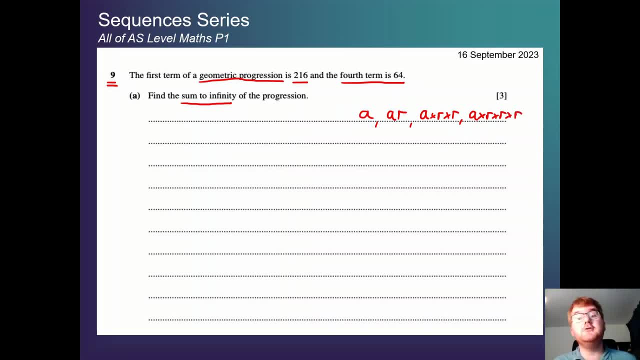 i R. So you can write any general geometric progression in this way. This simplifies down to A A R. Remember: R times R is just R squared, and R times R times R is just R cubed. So the first four terms of any geometric progression can be written in this way. We're told that. 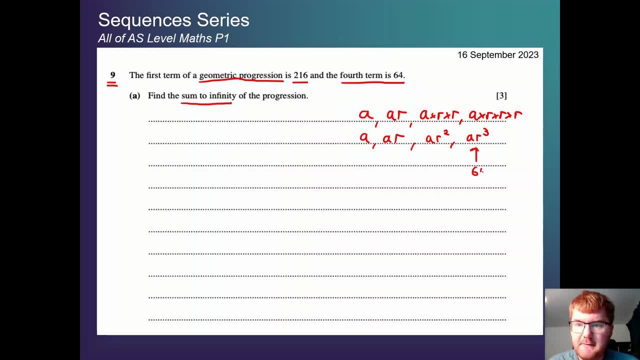 this fourth one here is equal to 64 and we're told the very first term here is equal to 216.. So if I take the fourth term here, so this A R cubed, this is equal to 64. However, we already know what A is. We know A is equal to 216.. Therefore, we can say 216 R cubed. 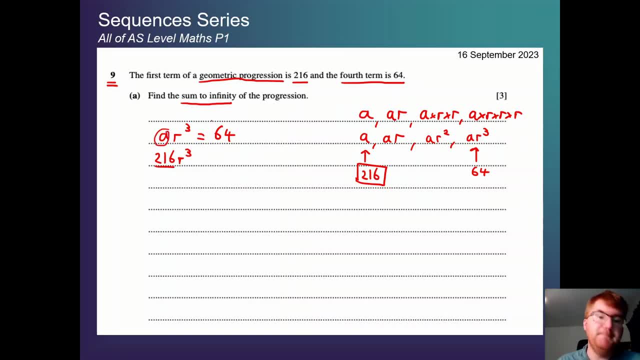 So we replace the R with the 216 is equal to 64. And this is now just a straightforward equation to solve here. So we're going to divide both sides by 216.. Remember, we want to get that R on its own as quickly as possible. This cancels giving. 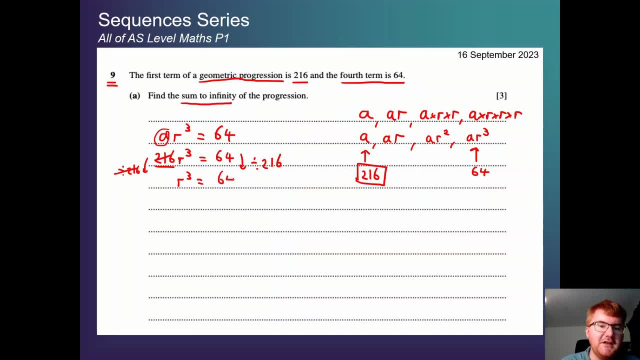 us R. cubed Again. fractions are the way to go here: 64 over 216.. So at this point, once we've got that, then all we need to do is then just work that down to our final answer. So all I'm going to do here is I'm going to cube root both top and bottom by cube root. 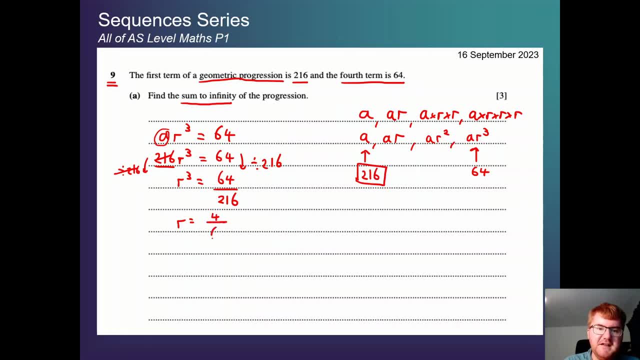 top and bottom. I'm going to get my answer of four over six, But again we can simplify that again down to two thirds again. So what we have to do is I'll just show you on the calculator. here is we just take the. 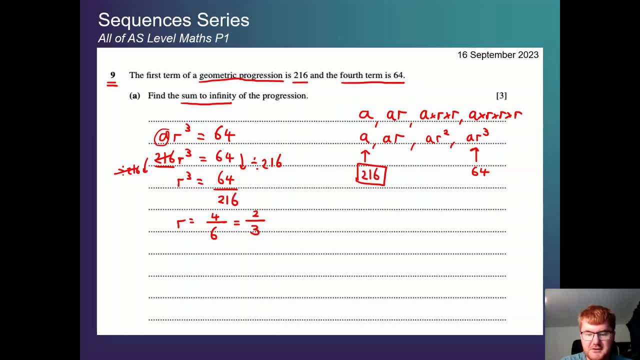 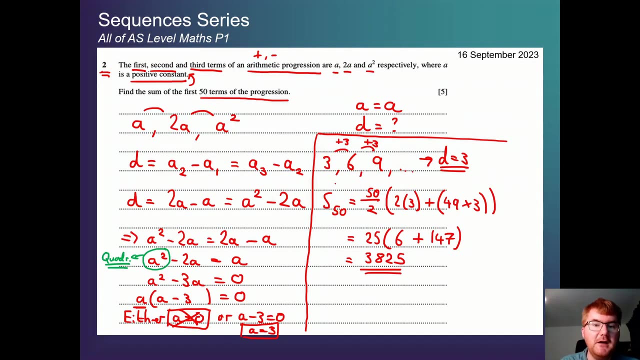 fraction or cube root of our fraction 64.. Well, calculator can just do this for you and see, we get immediately to the answer of two thirds. Now we know what this common ratio is and we know the first term. We can now use this formula. 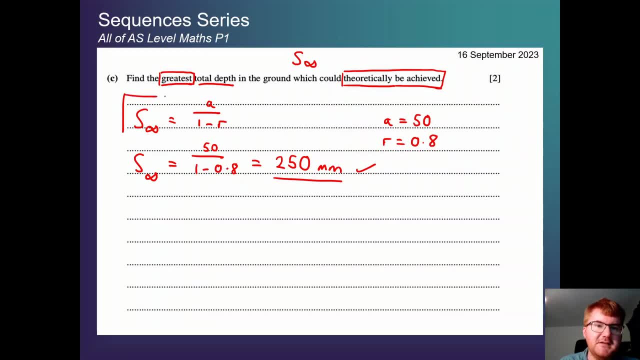 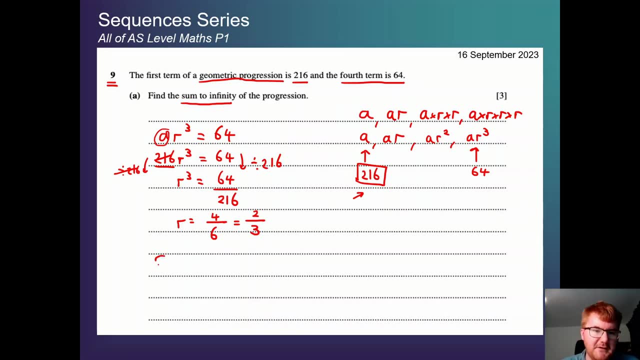 Okay, So what we've seen before, this formula here. so this S infinity is equal to a over one minus R. So now I'm just going to copy that formula down: So S infinity is equal to a over one minus R. Our first term here is 216 divided by one minus two thirds. Again, let 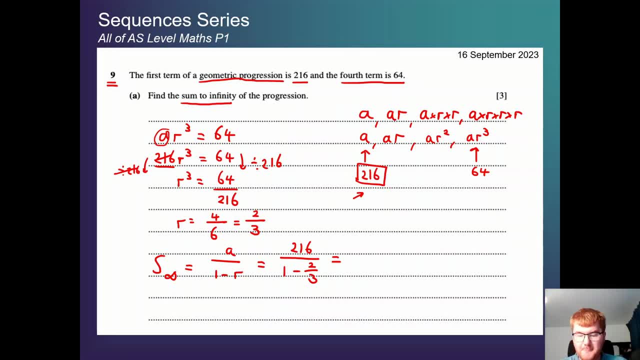 the calculator. do the mental maths for you. That's what it's there for. So 216 over one minus two over two thirds, So 216 over three. We pop this in and we get our final answer of 648.. Please use that calculator. 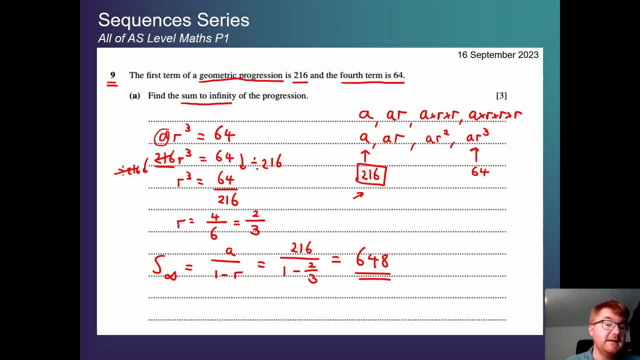 wisely when you're going through. Sometimes you'll need to simplify And again, if you've got something like this, just put it into the calculator, let it do its stuff, And you can always double check with some mental maths as well. That's perfectly fine. 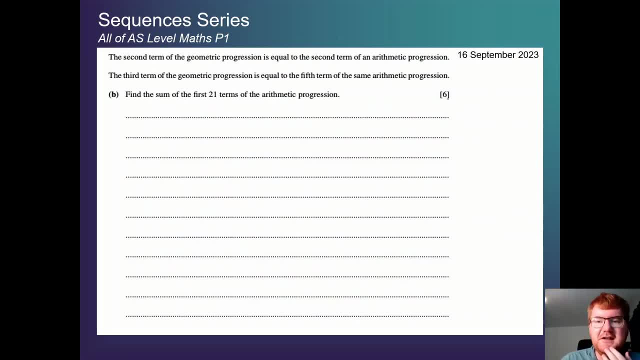 Onto question B, And this is where it gets a bit tricky Again. as soon as you see a six mark question towards the end of the paper, you need to think about this quite carefully. So let's read this through: The second term of a geometric progression is equal to the. 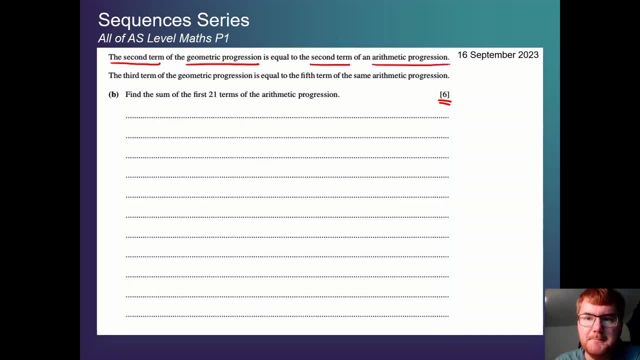 second term of an arithmetic progression. Now remember how we wrote out a general geometric progression: A, a, R, a R squared, a R cubed, and so on. We can do exactly the same for an arithmetic progression, because we're just adding or subtracting each time. So our first 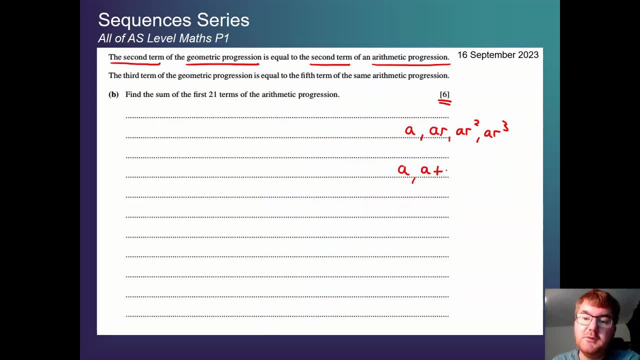 term would be A. The second term is just A plus whatever the difference is. The third term would be A plus two, lots of the difference: 2D, A plus 3D and so on. So this here. this is useful for your notes, so make sure if 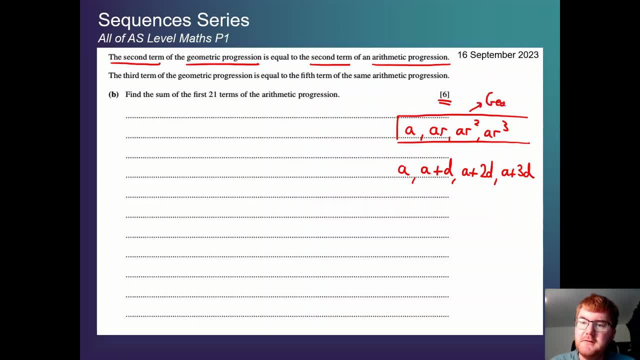 you need to go through this, write this down. this is geometric, here multiplying each time, whereas here this is arithmetic, also known as linear sometimes. so very useful notes to have. So, if I take the instructions from the question, the second term of the geometric 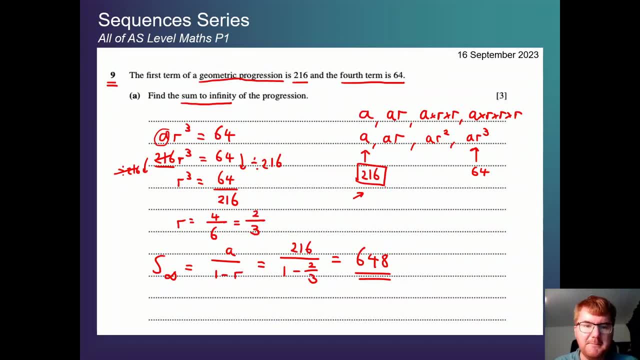 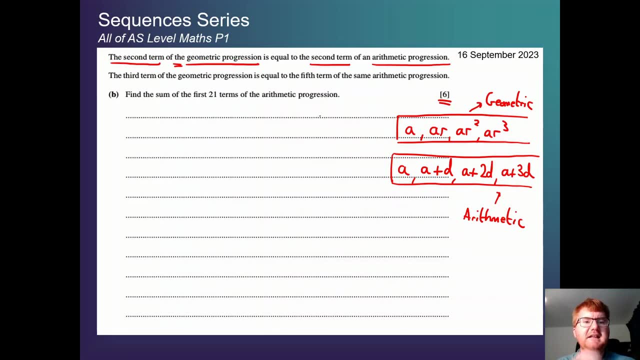 progression. so when they say the, it is what we've just been doing. so R is equal to two thirds, A is equal to 216.. So what this is saying here, the second term of the geometric progression, so A times R. so with this one that we have, it's 216 multiplied by two thirds. 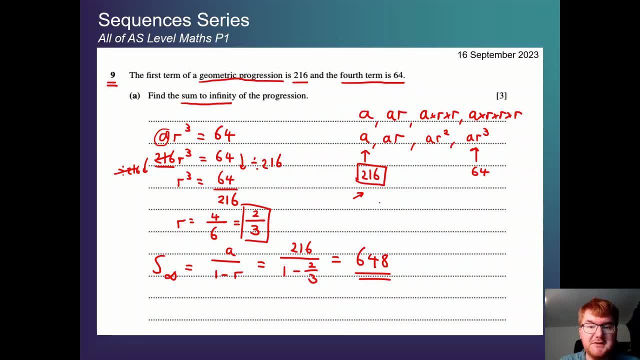 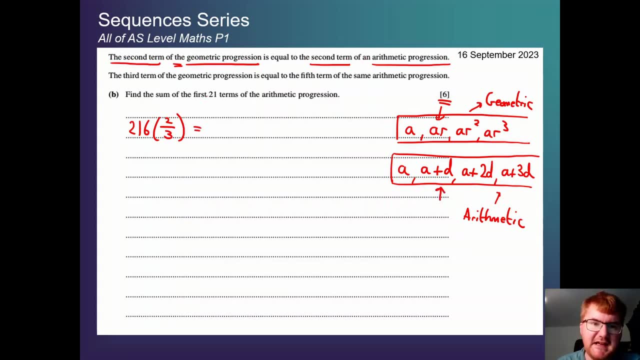 If you're wondering where those numbers come from, they're coming from the previous part of the question And this is equal to the second term of the arithmetic progression. so this A plus D, So these two things are equal to each other. We do a very similar process for the next. 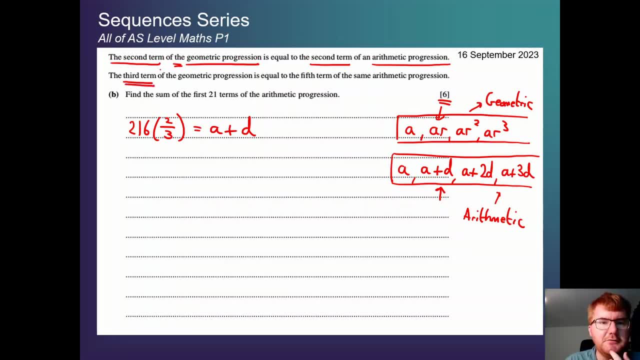 one. So the third term of the geometric progression is equal to the fifth term of the same arithmetic progression. So the arithmetic progression is the same top and bottom here. So the third term is going to be A, And that secondpo hundreds divided by R is circa A plus D. 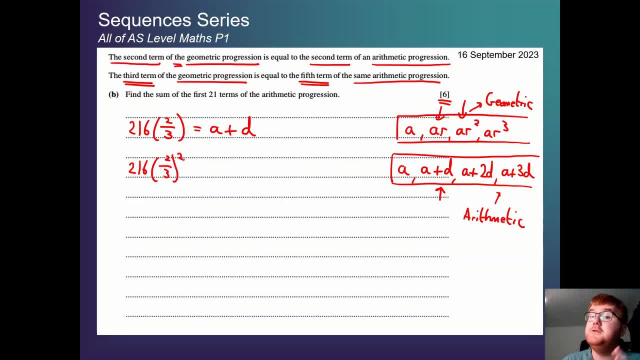 So thellä, we have a R squared here, so we have 216 and two thirds squared. Remember using part a here- And then the fifth term of the same arithmetic progression. Well, we've got the first term, second term, Third term, fourth term. So our next term would be A plus 4, lots of D. So 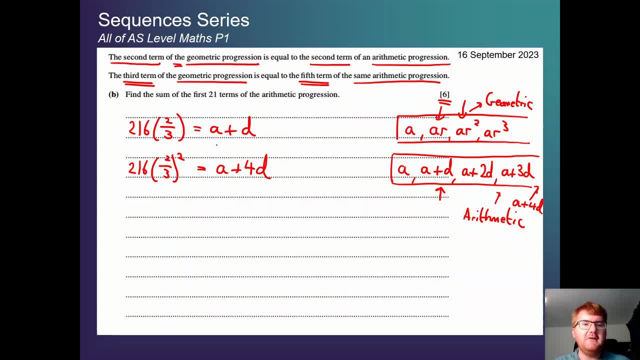 we pop that in Like. so Now we're going to do some work of our calculator, two thirds again. we're going to use a calculator to do this for us. and what do we get if we pop this in? we get 144, so we can say that this is equal to 144. a plus d is equal to 144 if we work. 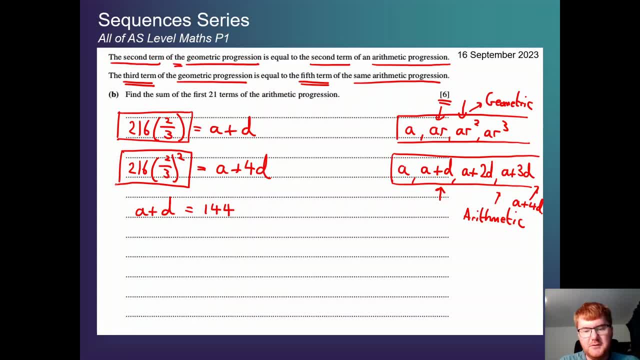 out what this is. in my next box i'm drawing, so we're just going to pop this over getting 96. so then we can say that a plus 4d is equal to 96. so i just worked out what this was, that i put the. 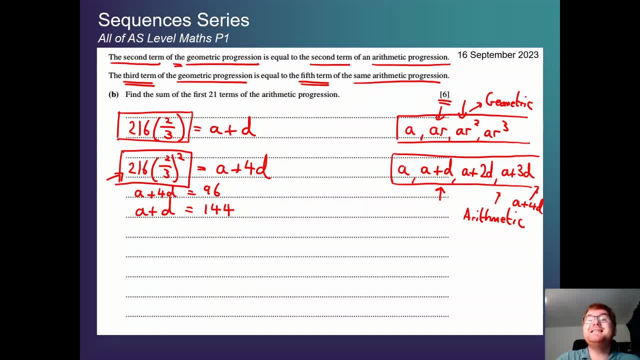 arrow to notice. we've got a very conveniently simultaneous equations- again an important skill on the igcse- and also a level course. so what i'm going to do is going to do it by elimination. i've set this up very nicely. i'm going to minus one equation from the other, so a minus a is zero. 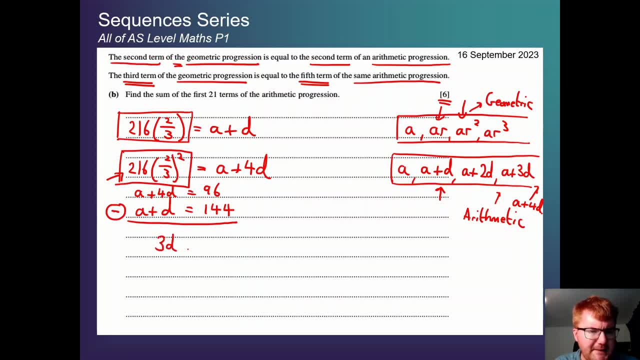 4d minus d is just equal to 3d, and 96 minus 144. if we pop this in, that gives us minus 48 and therefore we'll deal on its own. so we divide by three on both sides. this cancels giving us d. 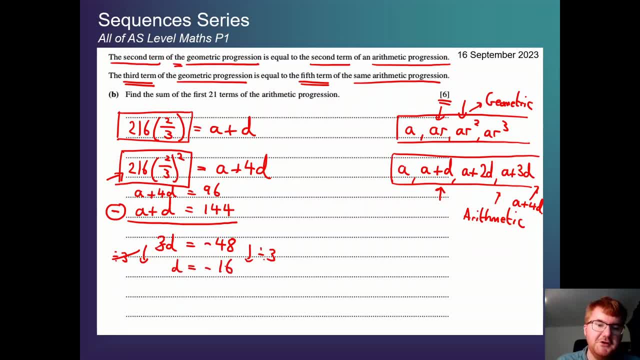 minus 48 divided by three. again, you can use a calculator if you so wish, but we then get minus 16. before we can work out the last part of the question here, we'll need to work out what the first term is. now we can use any of the equations we've seen so far. 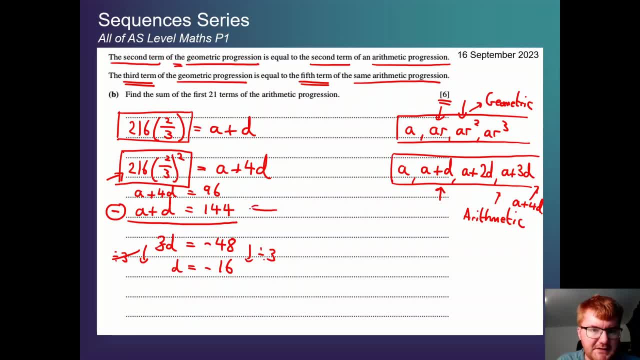 i think in this case i'm going to be using this one, so we're going to sub in one. so we've got a. wherever i see a d, i can now put minus 16. this is a very straightforward equation and therefore, adding 16 on both sides, we get a is equal to 160. now you're probably. 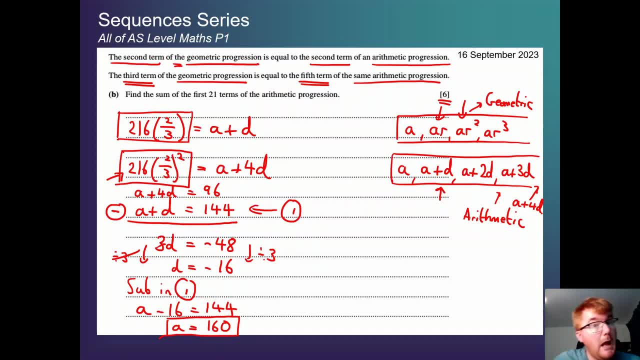 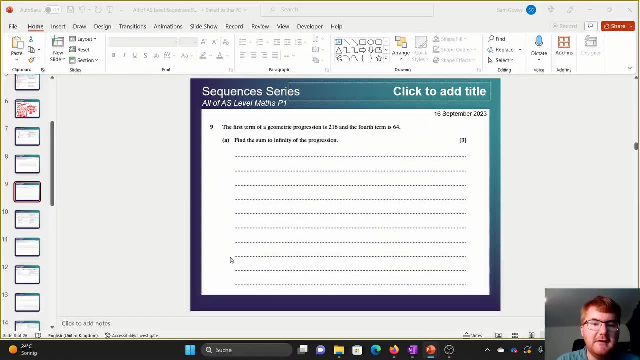 thinking at this point: oh, that's a lot of work to get the six marks, but we're not finished yet. so we have the sum of the first 21 terms to find of the arithmetic progression. this is why we spent so much effort working out the first term and the common difference. so let me create a new slide so we have a little. 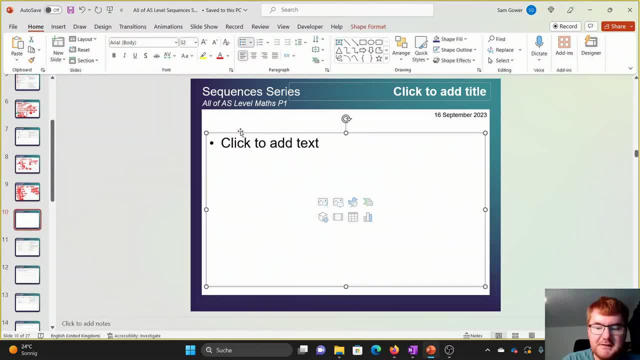 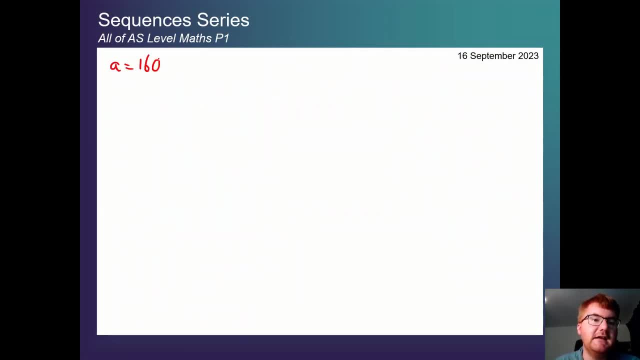 bit more room to work out the last part. so just to remind ourselves, we have: a is equal to 160, d is equal to minus 16 and we want to work out the first 21 terms. so our n here is going to be 21 and 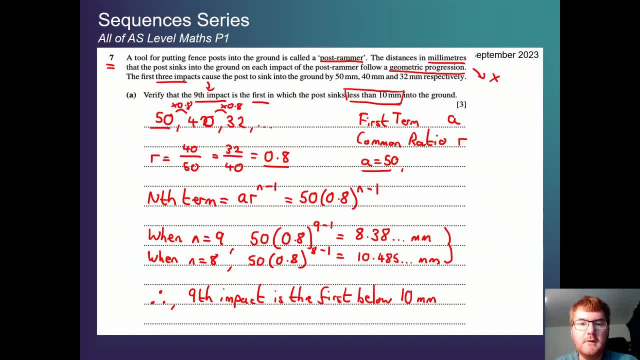 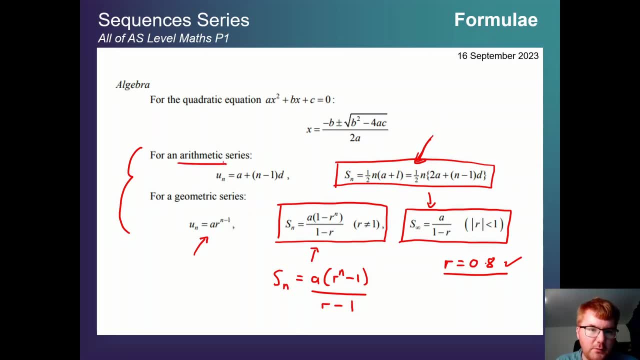 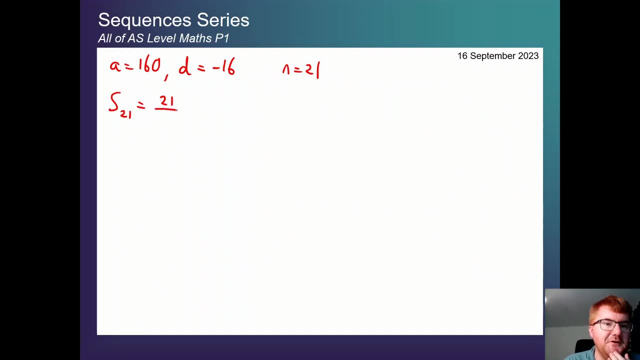 because arithmetic go right back to the start. here there we are. we're going to be using this formula over here, so we'll be using the arithmetic one, not the geometric. so if we pop this in, let's pop the numbers in see what happens. so we get 21 over 2- 2 lots of a. so 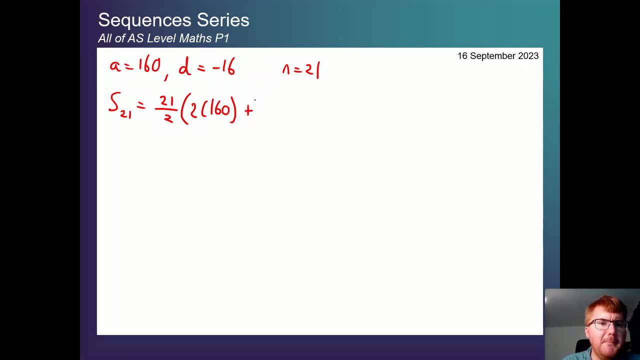 2, lots of 160.. plus n minus 1, so 1 less than 21, that's 20 times minus 16 again. you could simplify this down if you so wished, or you can just cancel. so you've got 10.5 here, 320. ah, this is helpful. 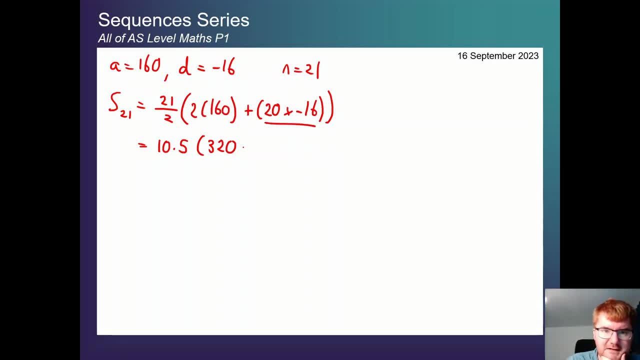 so 20 times minus 16 and if we work that out that's minus 320. so that means we're going to get 10.5 times 0, and anything times 0 is equal to 0.. so after all that effort for those six marks, the answer is just 0. that's what it was at. 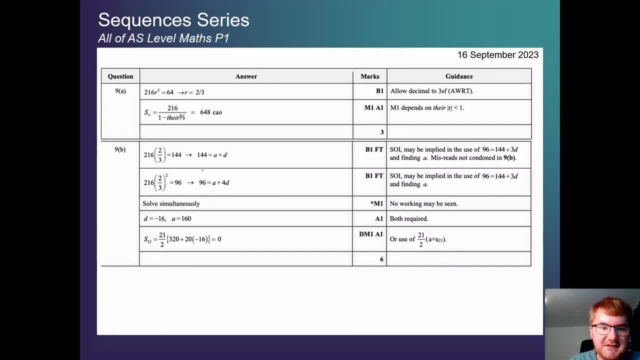 the end. okay, you can have a look through the mark scheme there. you can see where I picked up these marks again. quite useful, just to write these down again, both required. so it's important to be very, very clear how you got to these answers. okay, and over to a more unstructured 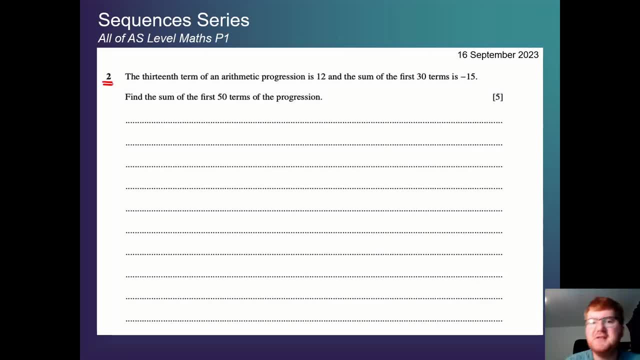 question. like we've already seen again. you can see question 2, question 7, question 9 does vary on the paper here. so the 13th term of the arithmetic progression is equal to 12. the sum of the first 30 terms is equal to minus 15 and from that somehow we need to work out the sum of the first 50. 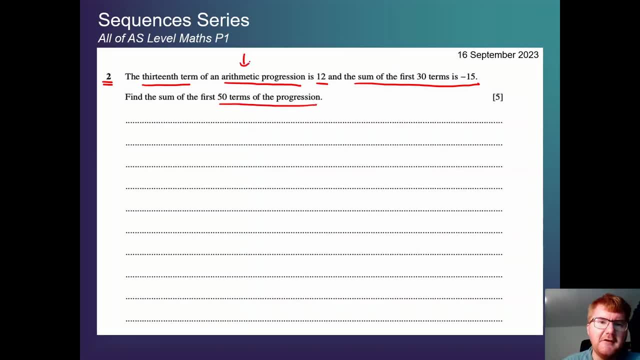 terms of the progression. so first of all is arithmetic. so if we wrote out a standard arithmetic progression, we'd have a a plus d a plus 2d, dot, dot dot. so we've got a a plus d a plus 2d, dot, dot dot. 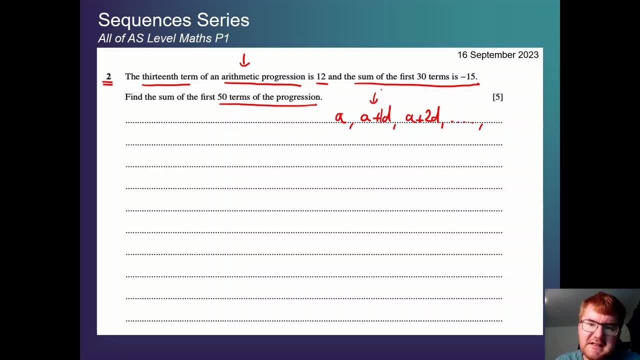 now notice here that a plus 1d is the second term, a plus 2d is the third term. therefore, if we want the 13th term, this number here is always one more than this term. notice this. so we're actually looking for a plus 12d here. notice the pattern here. if I did the fourth, 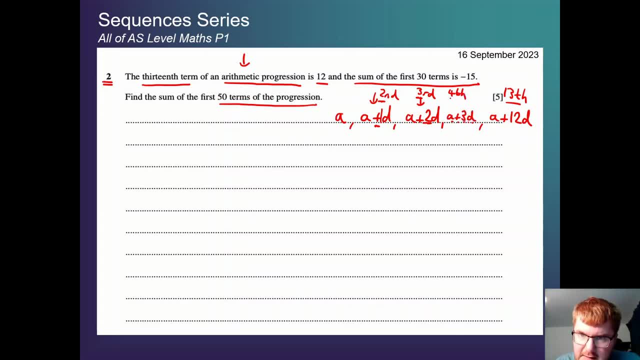 term, this would be a plus 3d, so notice the pattern. this is why the 13th term is equal to a plus 12d, so we can write this down so a plus 12d. my first bit of information is equal to 12. now this is a bit more complicated. here the sum of the first 30 terms is minus. 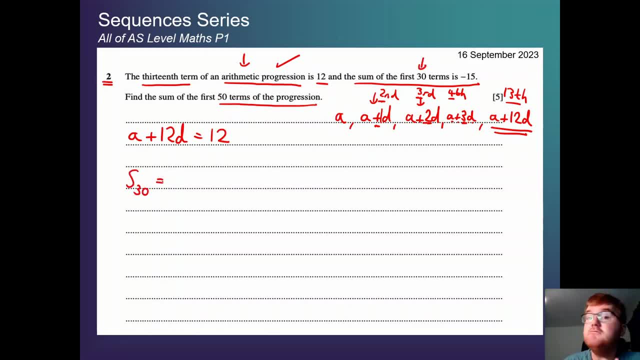 15, so s 30, which we can start using the formula at this point. so we have 30 over 2, two lots of a now n minus 1, one less than 30 is 29.. 2a plus 29d, so we're supposed to be able to divide this by 15.. 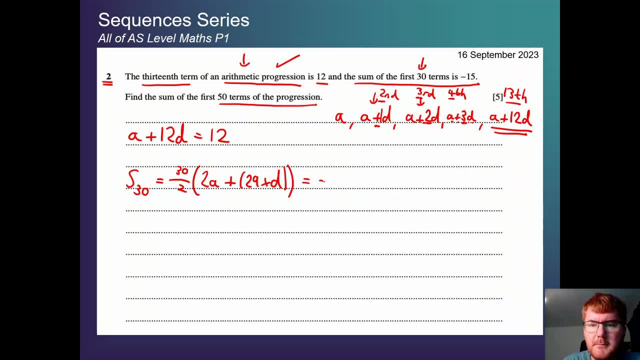 so we've got a 15.. so let's go back here and I'm going to divide this by 15 here, and that's because we need to divide this by 15.. so the way we do it is by dividing this by 15. we divide this by 15, by 15, divided by 15. 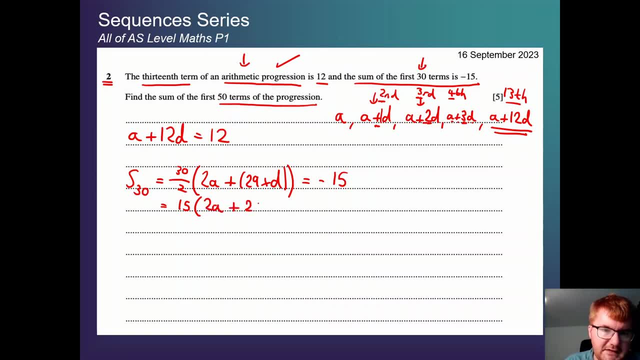 okay. so we need to do something like this: we're going to divide by 15, by 15, divided by 3.. so that's going to be a plus 5d. we're going to divide by 15 by 3, and then you're going to be able to a plus 2d divided. 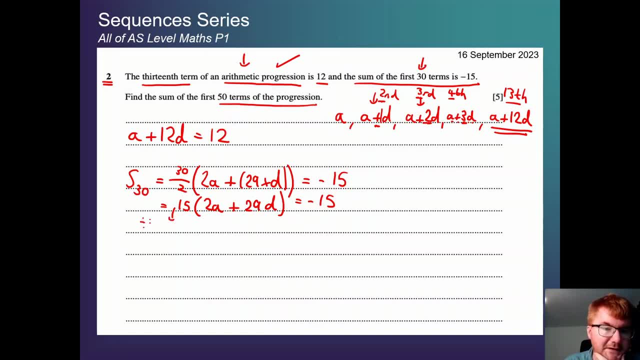 by 15 minus 2d. my first extends, so that's fine on both sides. always look for these opportunities to simplify, if you can. this cancels, leaving us with the bracket. so 2a plus 29d and minus 15 divided by 15 is equal to minus 1. okay now if 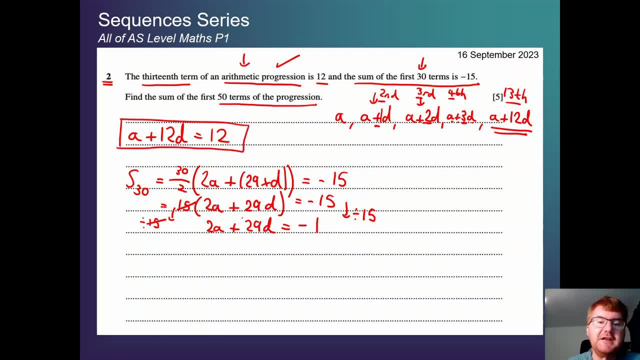 I wrote this equation underneath and tried the elimination method. notice doesn't quite work at this point because we have a 2a and an a. so before I write this down, you see, it's fine to make mistakes. you see, this is why I show you these typical mistakes and then how to think about it. 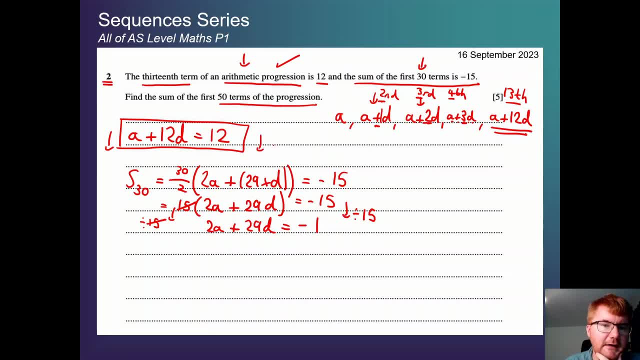 afterwards what I can do here. to be quite sneaky, I can times by 2 on both sides. perfectly fine, as long as you do the same thing to both sides, that then gives us 2 lots of a plus 12 times 2: 24d. 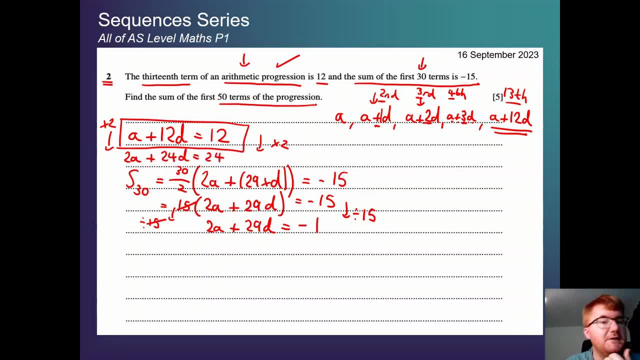 is equal to 12 times 2, which is 24. so I'm going to pop that underneath. now notice I can use the elimination method directly, which is very, very helpful, rather than trying a substitution approach or something else. so now I can just minus one equation from the other. 2a minus 2a cancels 29d minus 24d is 5d minus 1- careful here. negative. 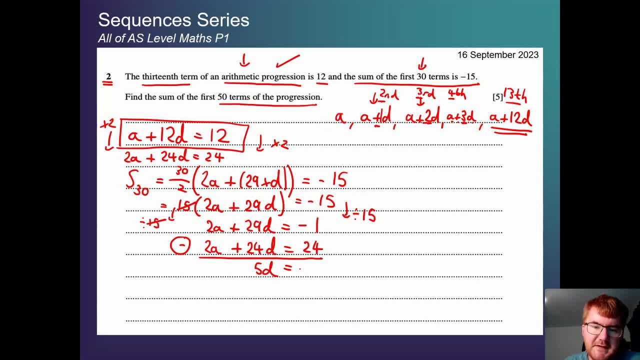 numbers. minus 1, minus 24 is minus 25. okay, and it's always a good sign, because now we're going to divide by 5 on both sides, because our common difference here is a whole number. if this is happening, then you're probably on the right track. again. it could be a 2.5, this is true, but usually these differences 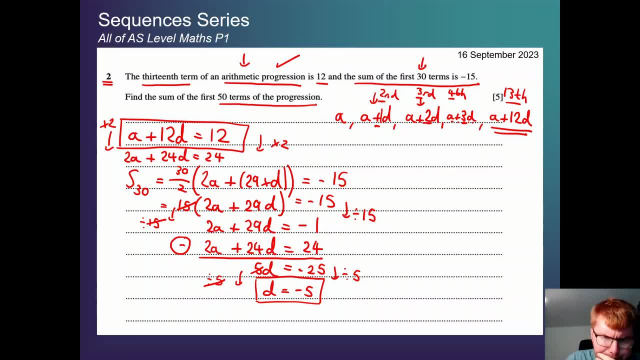 are generally whole numbers on this paper. so now we know d is equal to 5. don't forget, here we want to work at a as well, so I'm going to substitute into 1 here. into 1. that means I'm going to copy out this equation here: wherever I see a d, I'm going to put a minus 5. 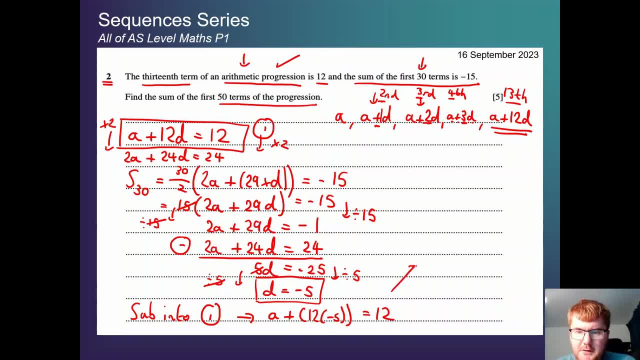 and this is just now a straightforward equation to solve. so we have: a minus 60 equals 12. therefore, a is equal to 72. so, just like before, we spent a lot of effort here working out the first term and the common difference of this particular problem. 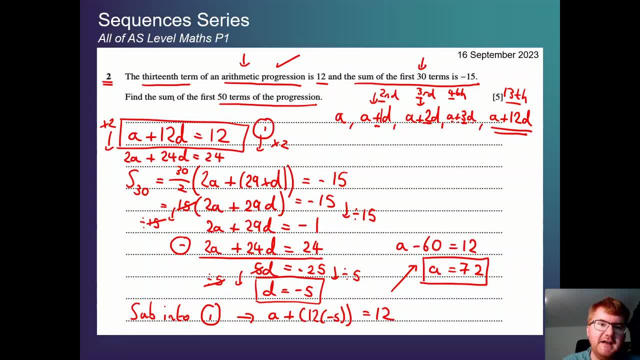 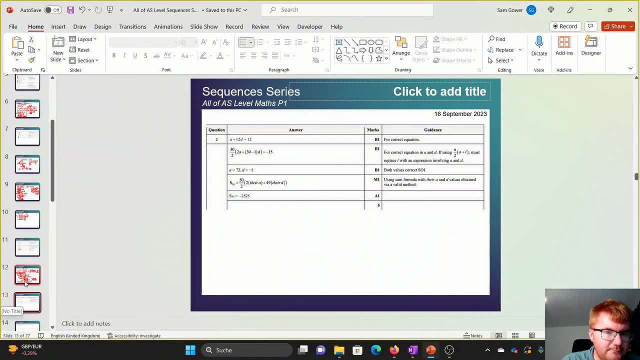 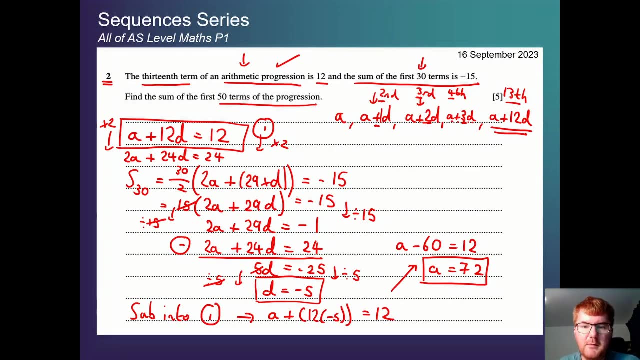 progression Again still not finished. for the five marks we still need to find the sum of the first 50 terms of the progression. So I think I need a little bit of room here to finish this question off. So let's write down the critical information here. So we 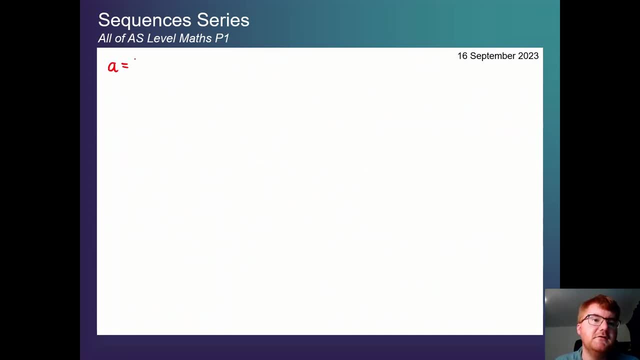 have. first of all, a is equal to 72, d is equal to minus five, and we want to work out s 50. Okay, so n is equal to 50. So if we pop this in s 50 is equal to 50 over two. 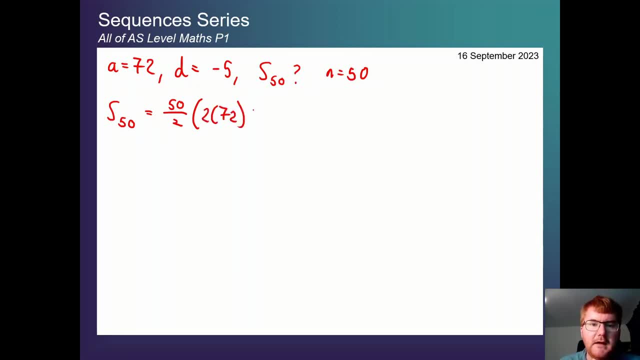 two lots of a, so two lots of 72, plus n minus one, so one less than 50,, 49, plus two lots multiplied by minus five. And this is a case where we can just put this in the calculator a bit of simplifying. So we get 25 here, 72 times two, that's 144.. That's not gonna be. 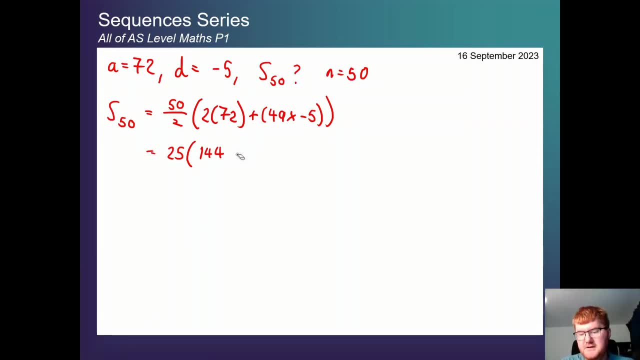 a plus, that's definitely going to be a minus 49 times negative five, So minus 245.. Again, we can just pop this straight in the calculator at this point or a little bit earlier. So both are absolutely fine. We get our final answer here: Minus 2525.. And that then gives. 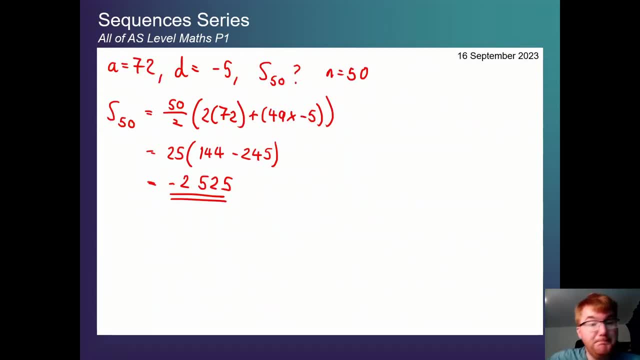 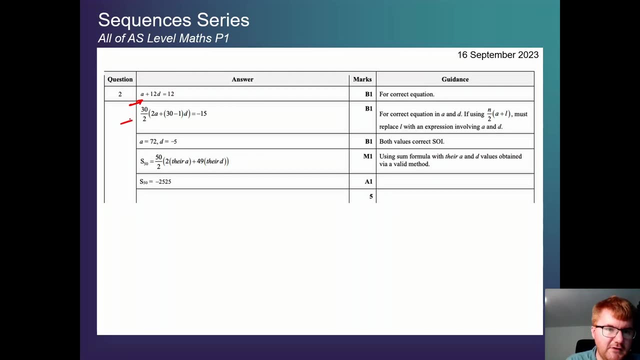 us all five marks for this particular question. Right, so you can have a look at the mark scheme. here Again, you can see all the different stages I've gone through. here Again: writing out this, writing out this, using that simultaneously to work out this part and then feeding it. 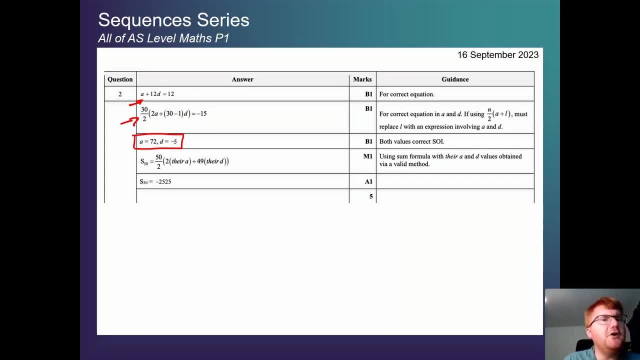 through to get these five marks. I do find out of the topics that I've talked about here, there's a lot of things that I don't want to talk about here. I don't want to talk about here. I don't want to talk about. 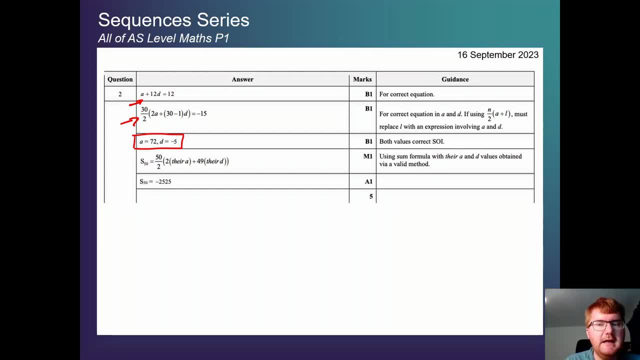 this particular paper one. It's one of the easier topics to really get a good understanding of quite quickly. So I really do encourage you to go through this video quite carefully and make sure you're getting all these marks on these fairly straightforward questions here. 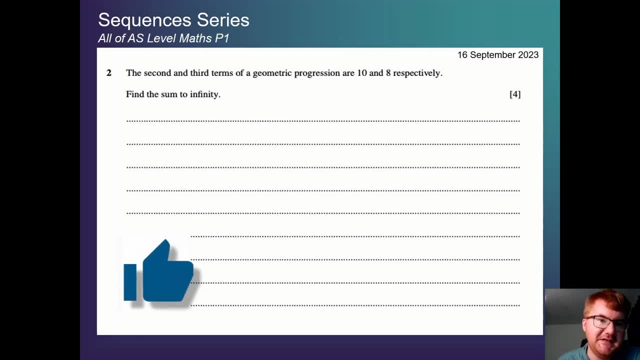 Okay, and on to question two here. So the second and third terms. let's underline that nice and carefully. the geometric progression. So remember we are multiplying each time. here are 10 and eight respectively. Okay, and then we need to find the sum to infinity. So again, we can think of this as: 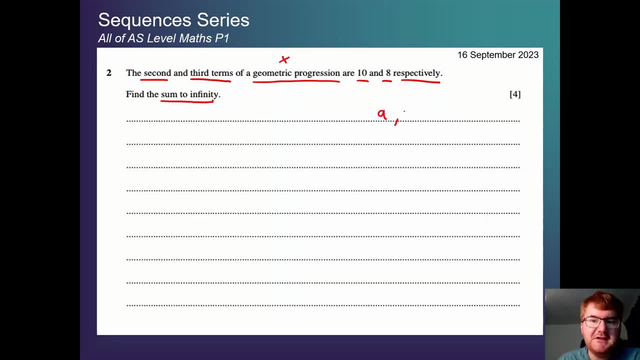 our first term. Now the second term of a geometric member is just A times R, And then the third one, as we've seen before, is A times R, times R or AR squared. So we're told here the second term- just to translate the question here- is equal to 10.. That's what it means. 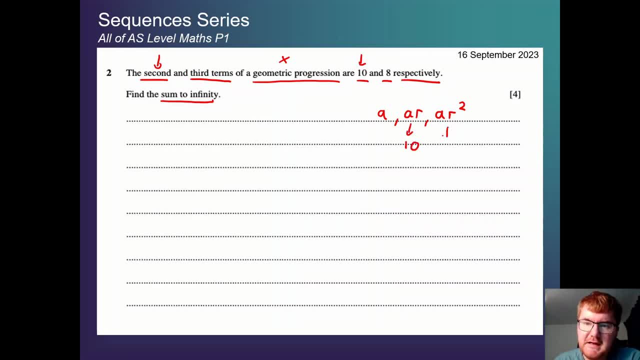 by respectively, And then the third term, that's going to be equal to eight. So we have here that AR squared is equal to eight, Whereas AR is equal to 10.. And we're going to see a technique we haven't quite seen yet. 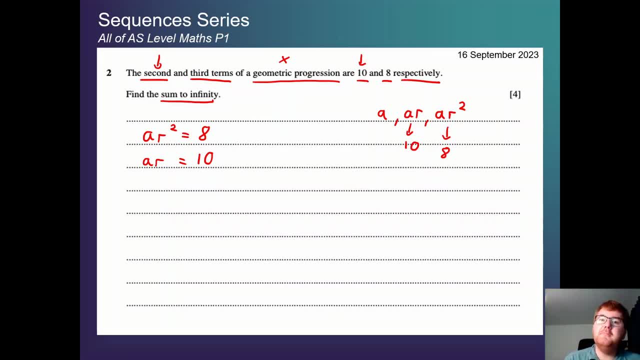 but still using this idea of elimination. Now, when we're doing arithmetic progressions, we took one equation away from the other. We can use a similar technique for geometric progressions. So what I'm going to do is divide one from the other. So if we go through this, 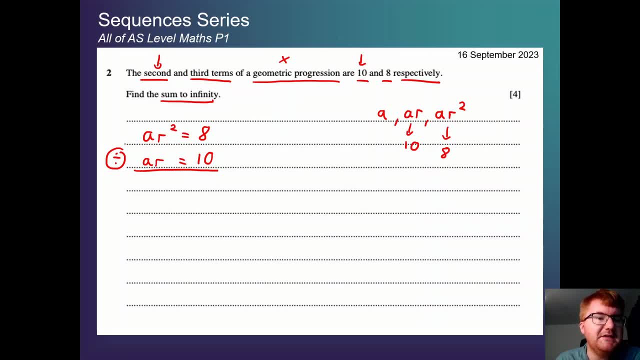 A divided by A is just equal to one. So if we divide by R to the power of one, that's just R. So think of this as R squared divided by R to the power of one- It's using our index laws here- And then eight divided. 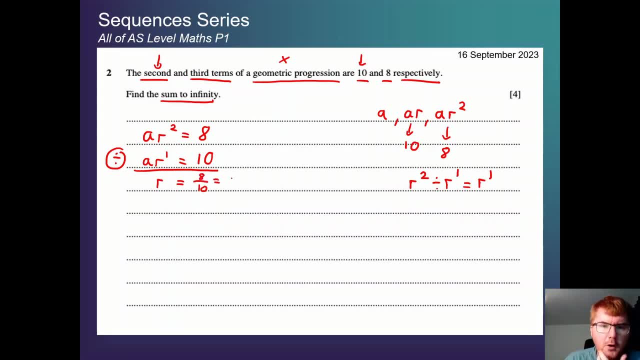 by 10.. Well, that's just eight over 10.. Or we can write this as a decimal or fraction of 0.8.. So now we know what R is equal to. We can now substitute that back in, So we're. 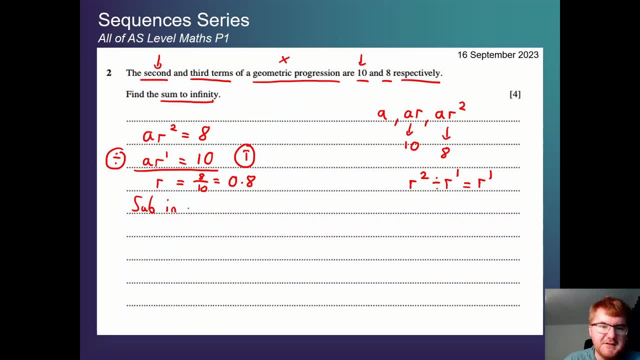 going to substitute into the easiest equation here. So substitute into one. So wherever I see, I see an R, here I'm going to put a 0.8.. So we get: A times 0.8 is equal to 10.. Therefore, 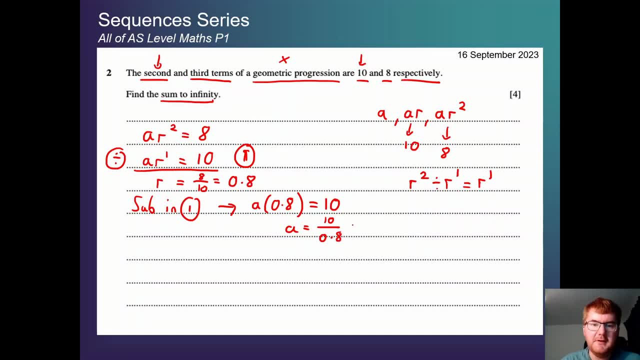 A is equal to 10 divided by 0.8.. Again, if you don't like that mental math, we can always pop this into the calculator. That's going to give you 12.5.. So now we know this A and. 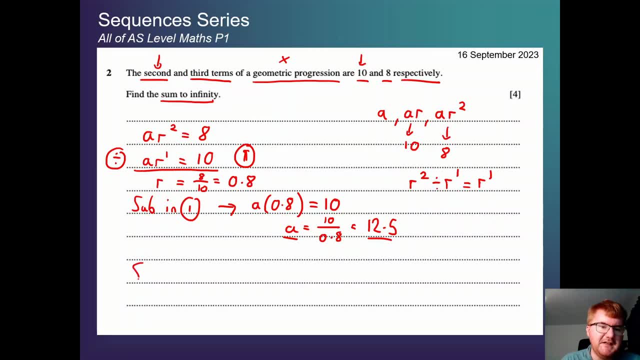 D or A and R. in this case, we can now use the sum to infinity formula Again. we've seen this a few times Now in the video. this is equal to A over one minus R. We pop in A, That's going to. 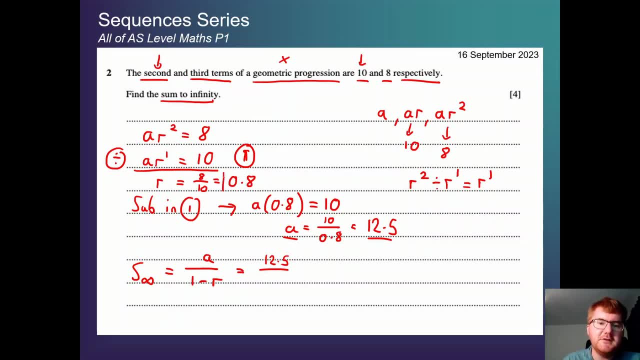 be 12.5.. We know R from previous question. previous part is 0.8.. So we have one minus 0.8.. Again, we just pop this into our calculator, Again, being nice and careful, making no typing. 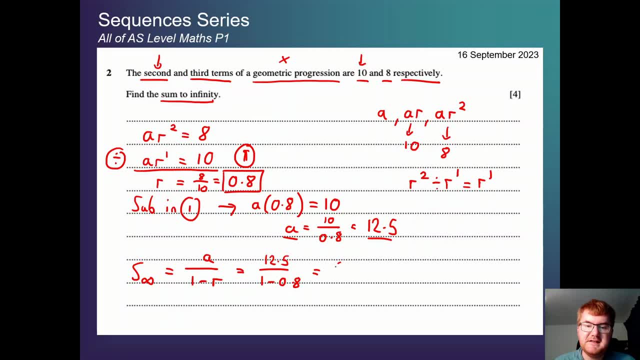 errors. And then we get our final answer of 62.5 as our sum to infinity Again. if you use fractions, you're going to get a sum to infinity Again. if you use fractions, you're going to get a sum to infinity Again. if you use fractions, that is also perfectly. 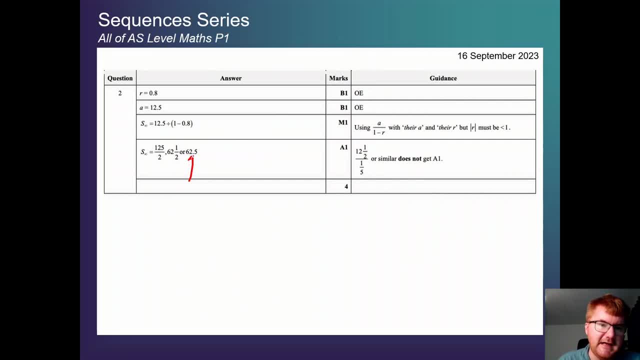 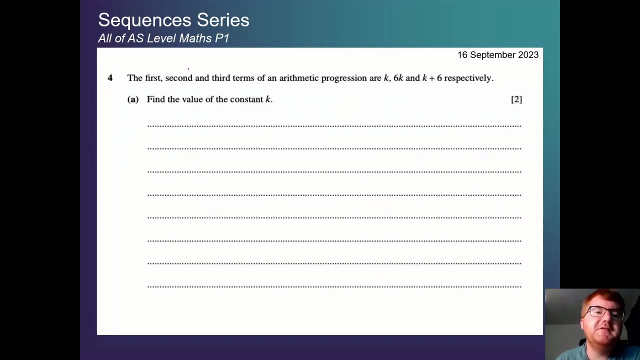 fine, So you can see the answer here. So again, you can have it in lots of different ways. My calculator gave it as straight away as 125 over two. That's also fine for all four. marks Onto our next question, slightly different to what we've seen so far. So the first second. 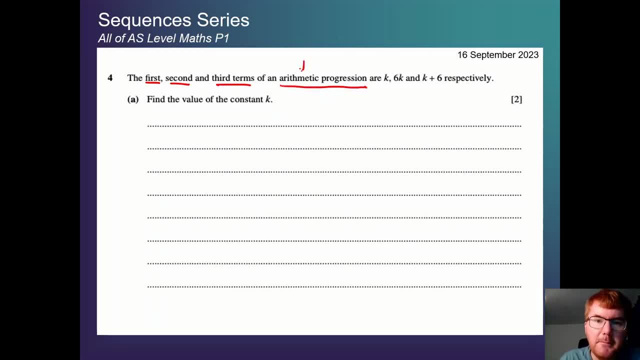 and third terms of an arithmetic progression. important word- so we're adding or minusing each time- are K 6K and K plus 6.. What are the terms? K 6K and K plus 6.. That's the last one. So the first, second and third terms of an arithmetic progression. 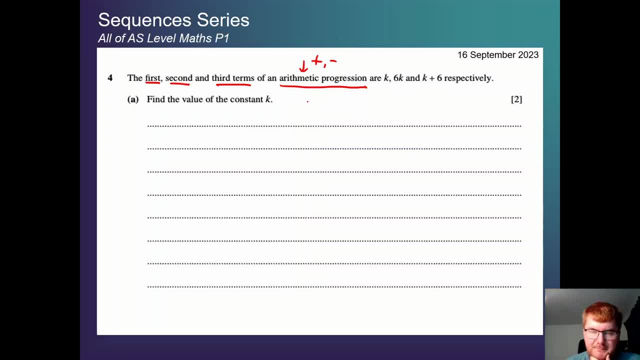 and we need to find the value of the constant k. Now we know what the first term is- that's just equal to k, but we don't know what the common difference is. But we can use a technique that we've already seen in this video. 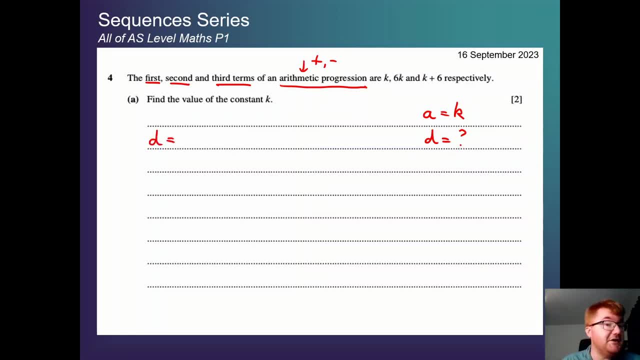 So the common difference is just say the second term, which in this case is 6k, minus the first term, which is just k, Or we can say it's the third term minus the second term, So k plus 6, the third term minus the second term. 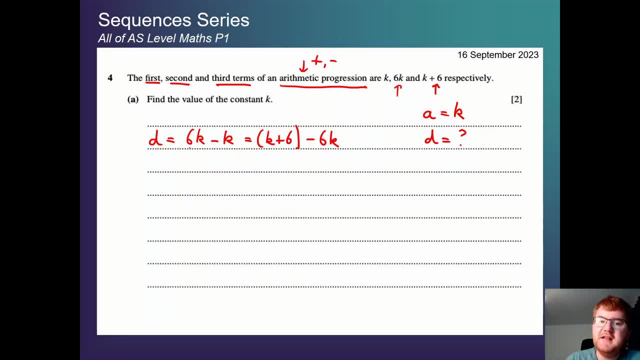 And notice, now we actually have an equation to solve because these two things must be equal to each other. So 6k minus k that's just 5k. Again, we can just write this out in full. So if we do a little bit of simplification here, 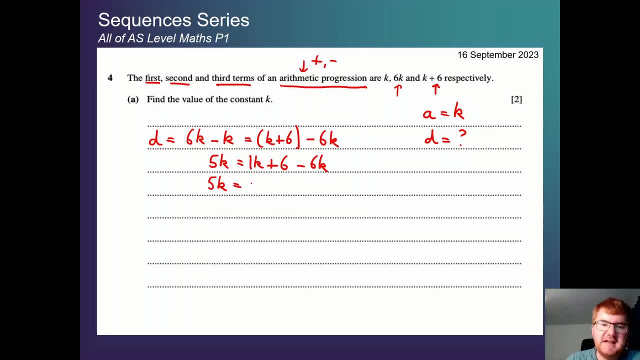 k minus 6k or 1k minus 6k is minus 5k. Again, this is just a straightforward. we're going to add 5k on both sides, so we get 10k is equal to 6,. 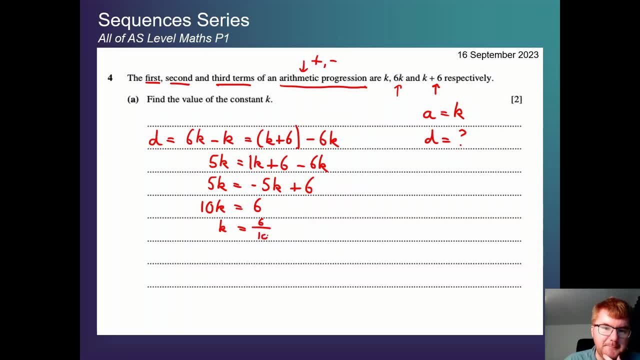 and therefore k is equal to 6 over 10, also known as 0.6.. So with this kind of question, again we're using that same idea of, if you want to work out the common difference, second term minus first term or third term minus second term. 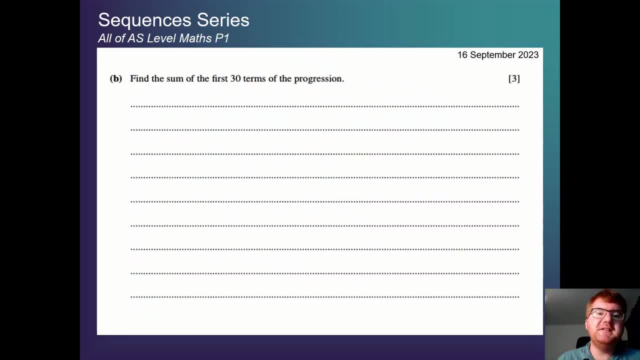 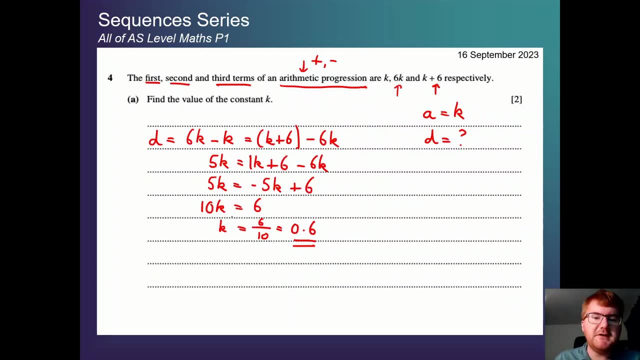 will do the job here. Now we need to find the sum of the first 30 terms of the progression. Now, before I do a question like this in this great exam technique, we now know k is equal to 0.6.. 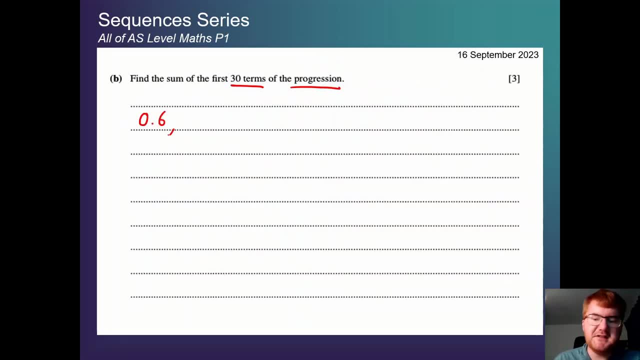 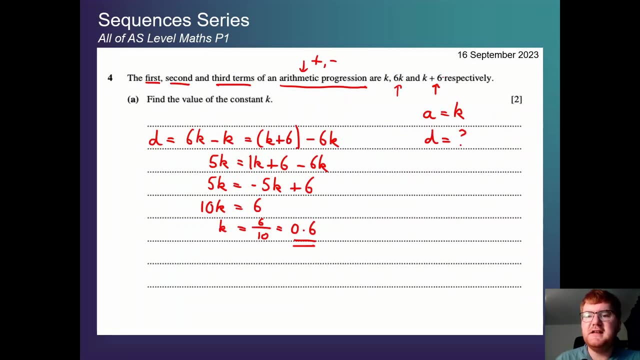 So if I write out this progression, we have 0.6, 6 times 0.6, for the second term is 3.6, and then k plus 6,. well, 0.6 plus 6 is 6.6.. 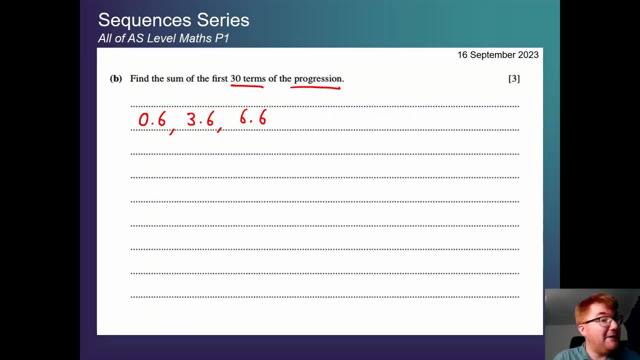 So before I do anything in this question, I'm going to check this is arithmetic before I try and get to these three marks. Notice it is because we're just adding 3 each time. so we've confirmed it is arithmetic and we haven't made a mistake in the previous question. 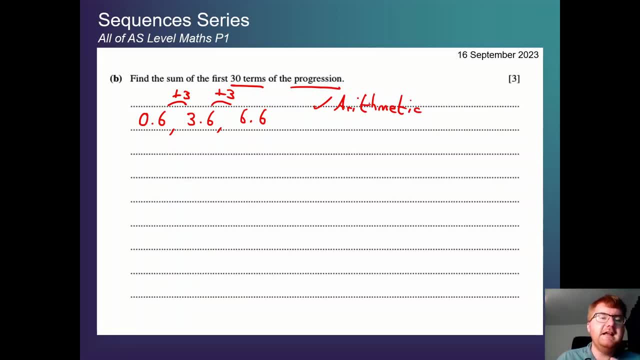 One of the worst things you can do on an A-level paper is you've got that answer but not double-check that it actually does do what it says. It should be arithmetic, because if you notice an error here you can go back and then try and find the right answer. 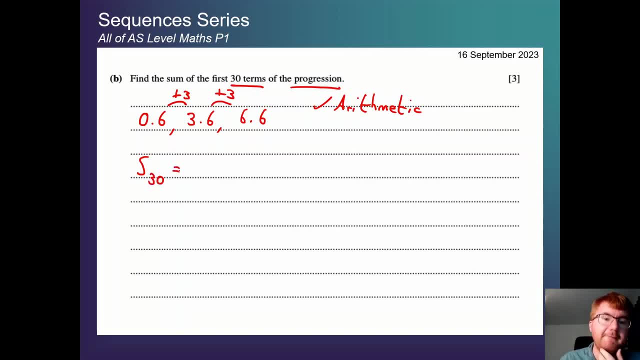 Now we want to find S30.. It's again using that formula we've seen before, So n over 2, so 30 over 2.. Two lots of the formula, So two lots of the first term, so two lots of 0.6,. 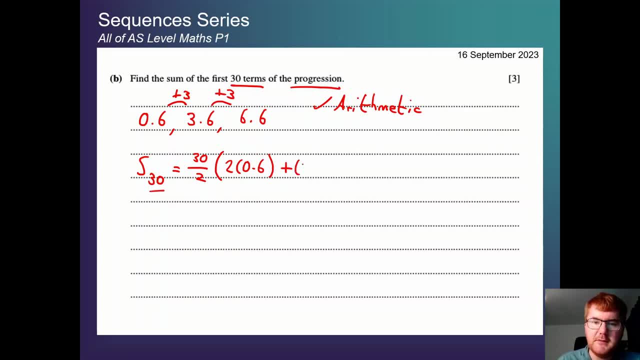 plus one less than n, so that's going to be 29, times a common difference which we just worked out, That's equal to 3. here Again, we can simplify this down, so we get 15, 1.2, plus 29 times 3 is 87.. 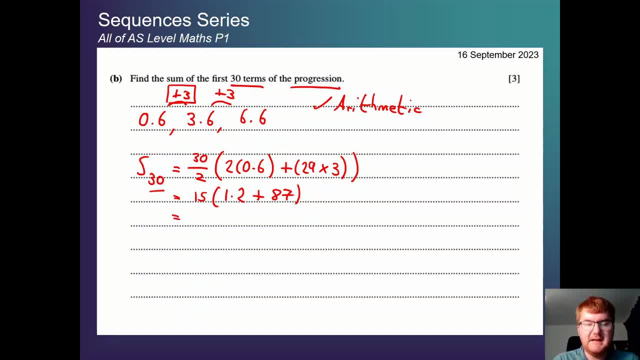 And if we pop the rest of this into our calculator, we can let it do. We can let it do the hard work for us. Now I'm getting my final answer. The whole number is always a good sign: 1,323.. 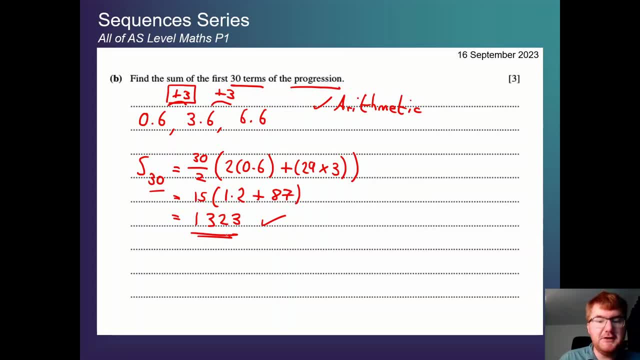 And that gives me then all three marks for this part of the question. Again, you can have a look through the mark scheme and make sure you're happy with what I've done so far, Hopefully by this part of the video. 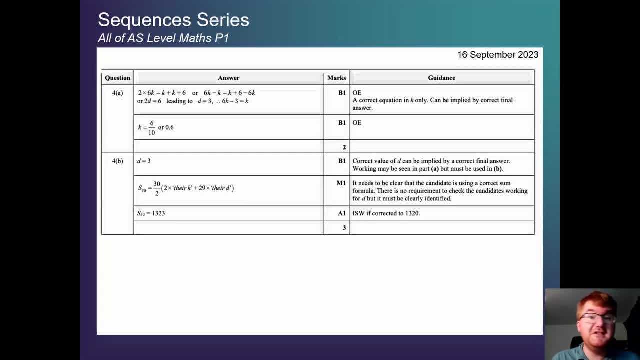 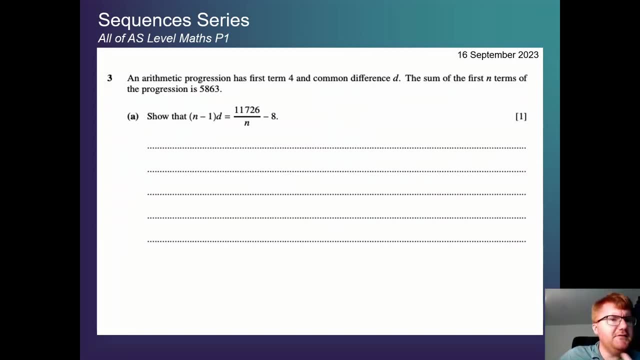 you are getting more comfortable with all the different techniques you'd need to have on this A-Level Maths Paper 1.. Now we have a slightly different style question. We're going to look at this one So, even though it's question 3,. 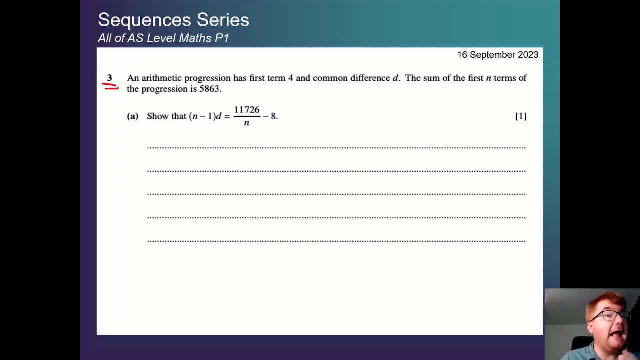 it's slightly strange in its construction and this can throw some students off. So we have an arithmetic progression. So again adding and minusing here, First term of 4.. So a is equal to 4. And the common difference is just d for the moment. 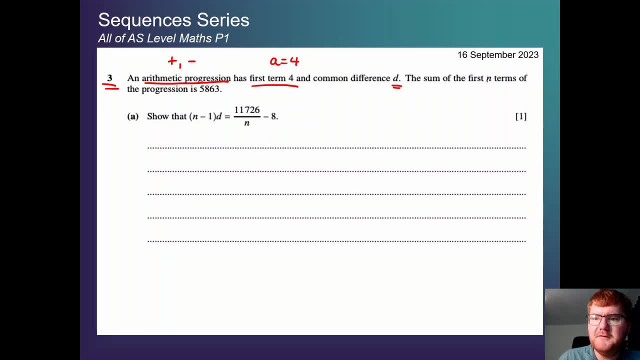 And the sum of the first n terms of the progression is equal to 5,863.. Okay, that's kind of strange. I mean to show this random thing. see what I've got here. So I'm going to show you this random thing seems to exist. 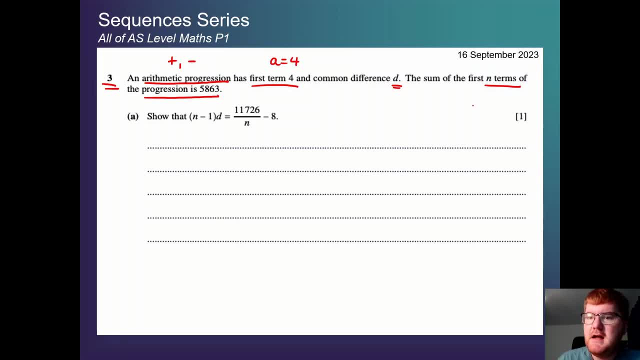 Now, the first thing I do with a question like this, I just write out the sum of the first n terms, So essentially, sn. we're just going to write the formula from right back at the start of this video. So we have n over 2,. 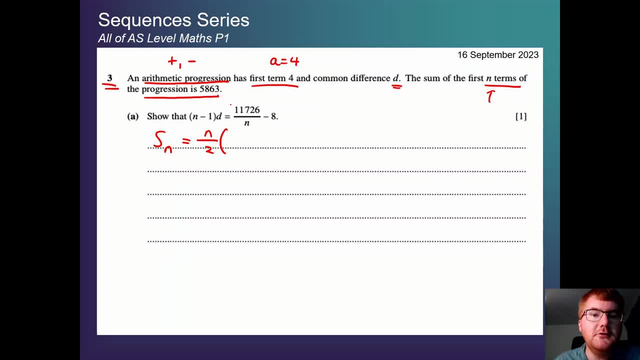 2 lots of a. However, we know what a is here. We know a is equal to 4.. So we have 2 lots of 4.. Now we don't know what n is, so n minus 1.. And we don't know what d is. 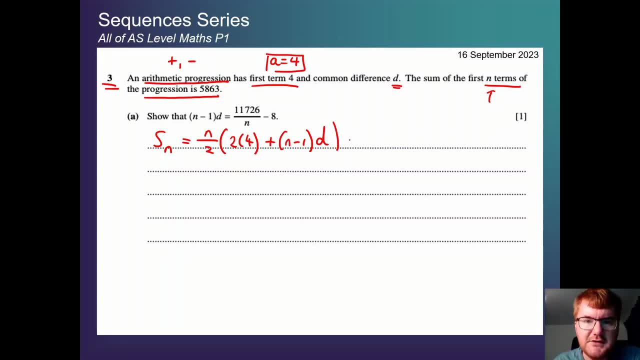 so we leave it as d And this whole thing is equal to 5,863.. Now this is a really important algebra technique. I see what I have here and I want to make it look like this. So essentially I want to make: 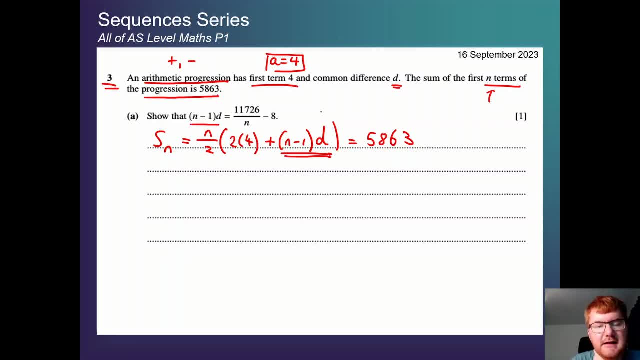 this n minus 1 d, the subject, This whole thing, the subject. Now, the first thing I can do here is just do a little bit of simplification. So 4 times 2 is 8. I'm going to definitely leave that n minus 1 d alone. 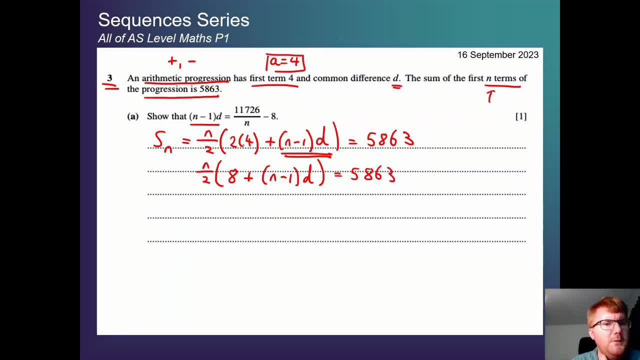 because that's what we want at the end. Okay, well, we can certainly multiply both sides by 2 to get rid of this horrible fraction, So that seems a thing to do. here Again, fractions generally want to simplify here, So we can cancel this out. 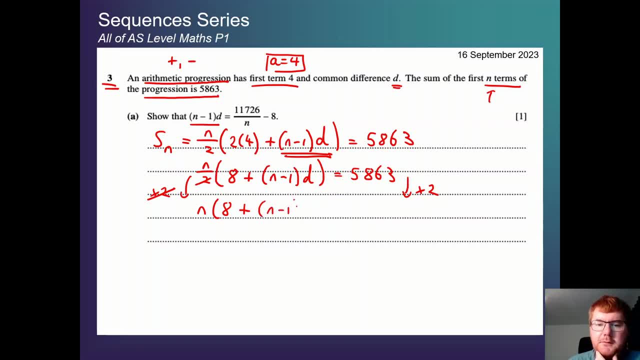 leaving us with n 8 plus n minus 1, d is equal to 5,863 times 2 is 11,726.. As soon as I see this- I see this in the question- I must be on the right track here. I'm not too far away. 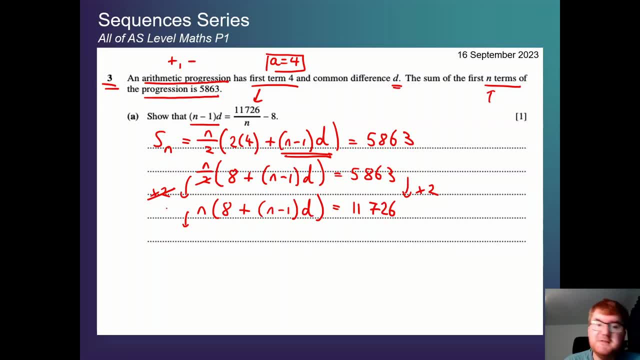 Now let's get rid of this n. So the opposite of timesing by n is dividing by n, It seems, slowly building towards what we need to show. This cancels, leaving us with 8 plus n minus 1 d, And we're. 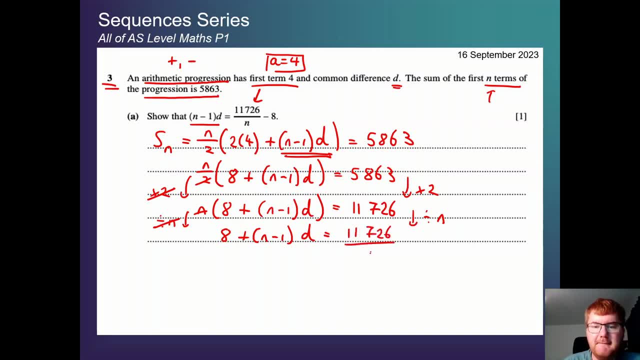 dividing by n. so we can just write this as a fraction, very close to what we need, And you can probably see at this point. all we need to do then is just minus 8 from both sides, And then we get exactly what. 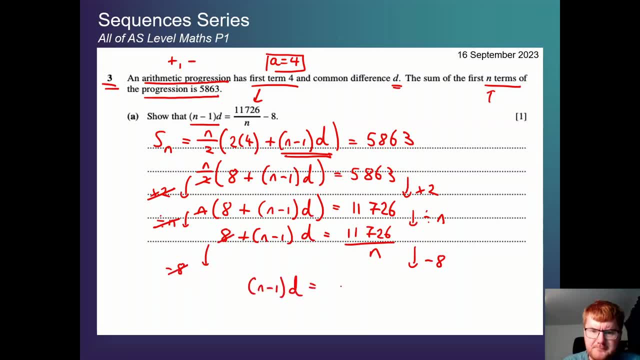 we are looking for. So n minus 1 d is equal to 11,726 over n minus 8.. Bit mean for one mark. to be quite honest, There's quite a bit of algebra to do there, But okay Again, as I said, 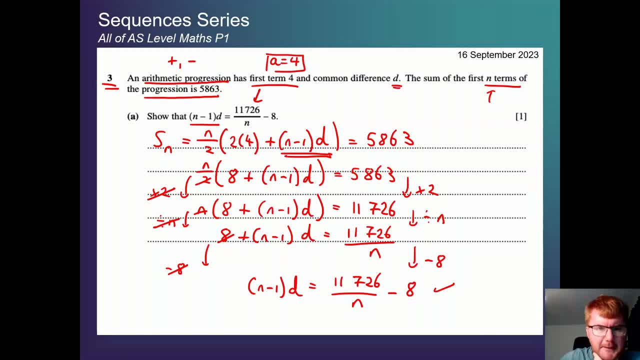 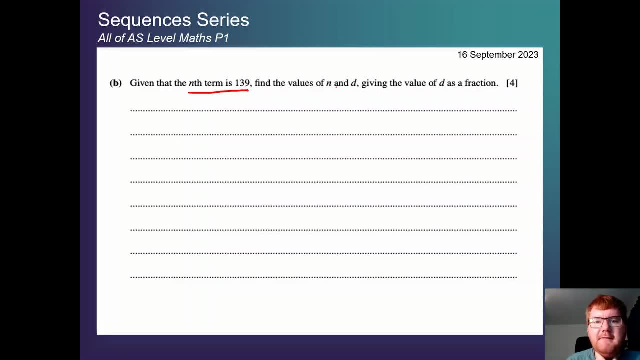 slightly strange question. This is why I've included it in the video Now, given that the nth term is 139, find the values of n and d, giving d as a fraction. Not much structure here to work with, but let's see what we're given first of all. 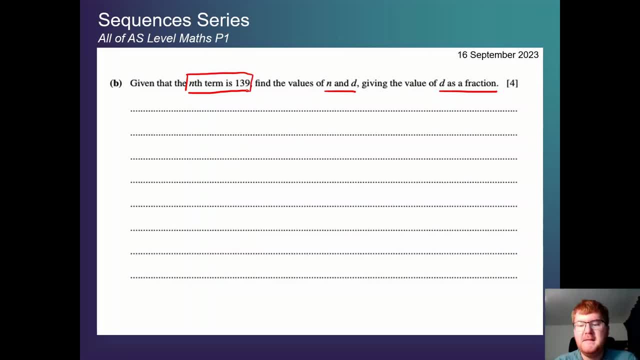 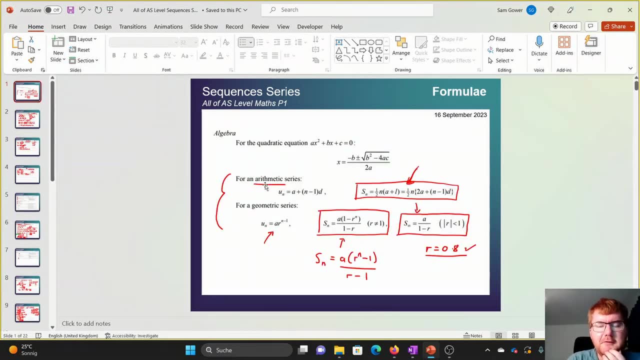 We're told, the nth term is equal to 139.. Now, if I go right back to the start- here we've gone through a lot of work today- The nth term for an arithmetic geometric series. you see this equation here: a plus n minus 1 d. 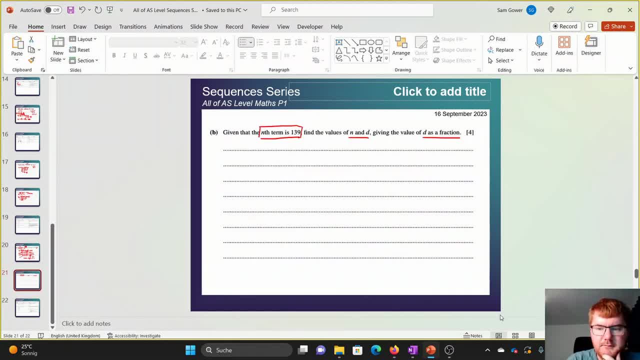 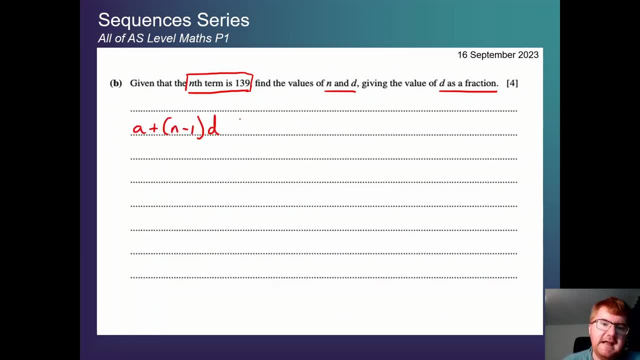 So what I'm going to write down is that a plus n minus 1 d the nth term- it says that on the formula sheet is equal to 139.. Now we actually know what the first term is. don't forget that. 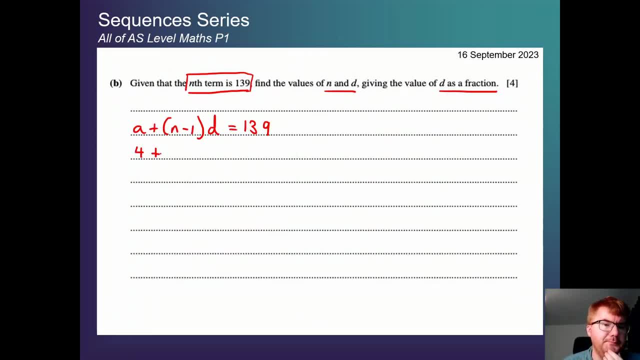 We know a is equal to 4.. So I'm going to pop in 4. And all I'm going to do is just subtract 4 here. You're thinking maybe y at this point, but that's fine: n minus 1 d. 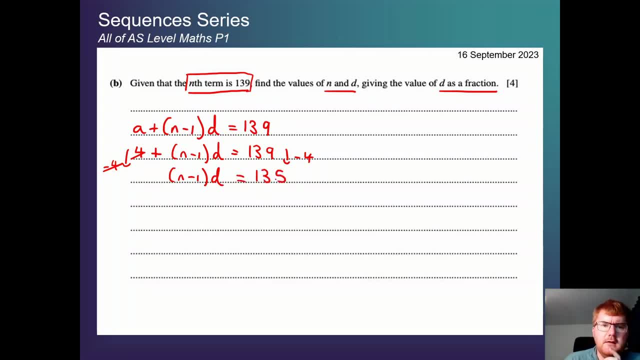 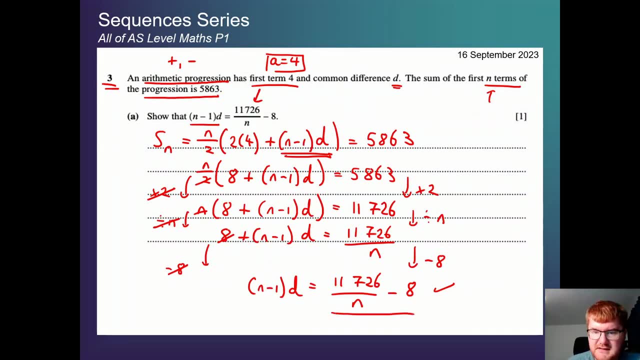 and that's equal to 135.. The reason is, we spent a lot of time in the previous question working out what n minus 1 d was. n minus 1 d was equal to this expression here, So all I'm going to do is: 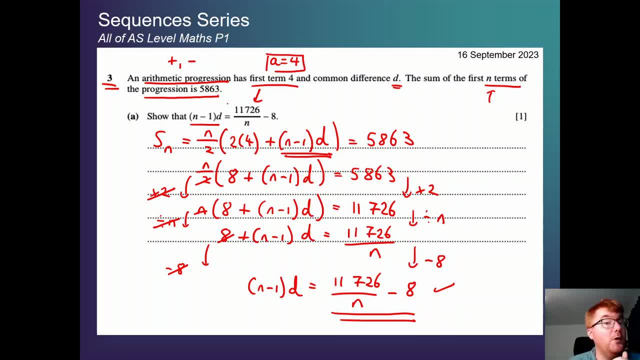 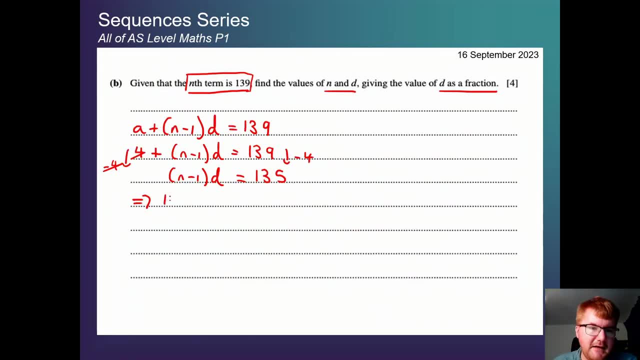 wherever I see an n minus 1 d, I'm going to replace it with what we know from part a. So all I'm going to do is replace that with the right hand side. So 11,726 over n minus 8. 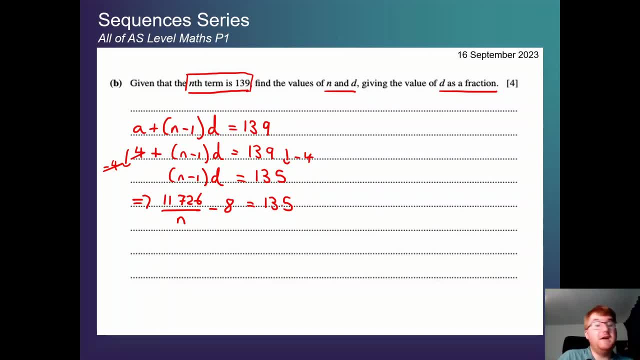 is equal to 135.. This is actually an equation that I can solve, Slightly unconventional, but certainly I can solve it. I can add 8 on both sides. That gives me then: 11,726 over n is equal to 135 plus 8. 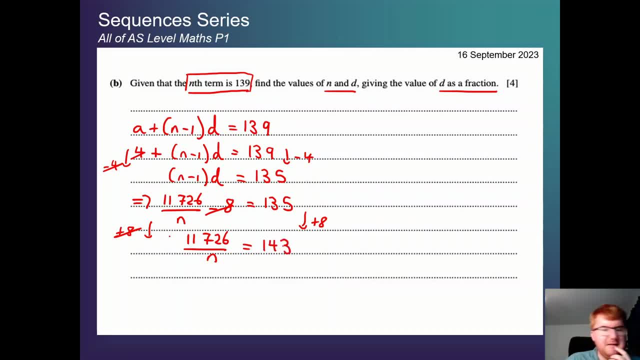 is 143.. Again, there's a couple of different ways you can do this. at this point. You've probably seen it from trig, but you can kind of flip these. Let's just do it in the kind of standard way. here I'm going to multiply by n. 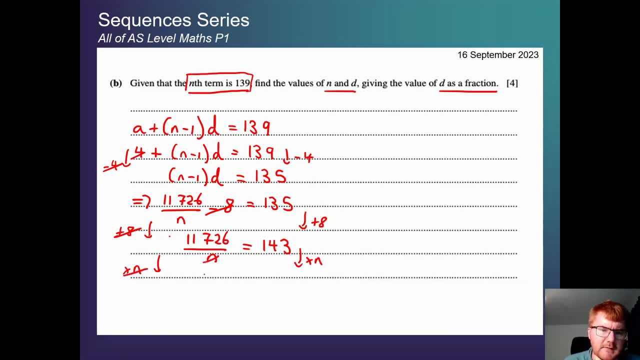 Again, if you can go straight to the answer, it's fine. So I get: 11,726 is equal to 143 n and then I divide through by 143.. If you do sine cosine and tangent, you see this idea a ton. 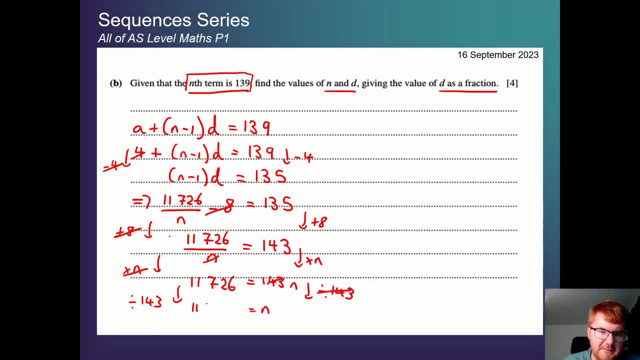 So this cancels, So we get: n is equal to 11,726 over 143.. And this is where we hope. this is a whole number, That's always a very good sign, and it is Therefore n is equal to 82..